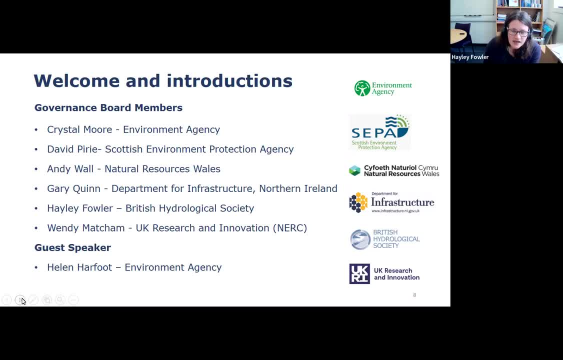 So the way it works is that the governance board contains a member from all of the regulators across England, Scotland, Wales And Northern Ireland. that's the Environment Agency, the Scottish Environment Protection Agency, Natural Resources Wales and the Department for Infrastructure Northern Ireland. 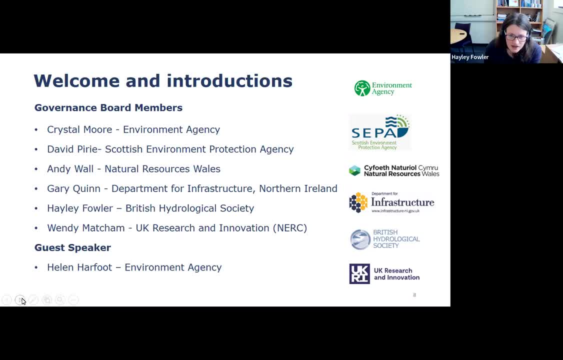 And then there's also a representative from the British Hydrological Society, And at the moment that's myself, and somebody from UKRI as well, And at the moment that's that's somebody sitting on from, from NERC and the governance board. really. 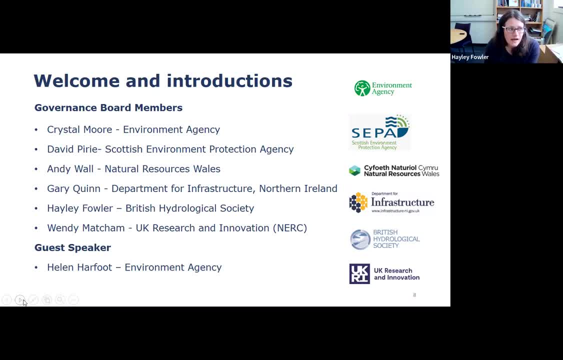 takes an overview of the roadmap, Of the roadmap programme and ensures that aligns the projects and the funding aligns with the roadmap and obviously providing an overview of the programme activities and commissioning projects where needed and also finding and providing the funding for those activities. as 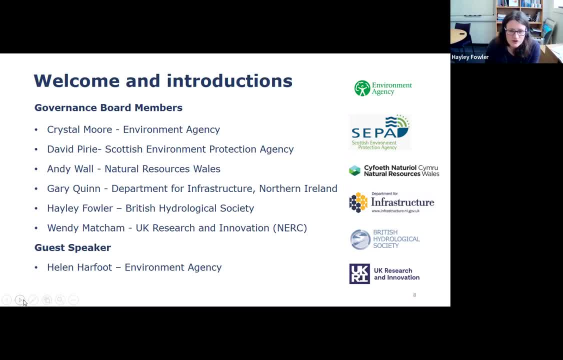 well as, in particular, the British Hydrological Society is providing support in terms of access to the community and comms and things like that and things like that. So it's very much a sort of you know joint or there's all parts of the UK. 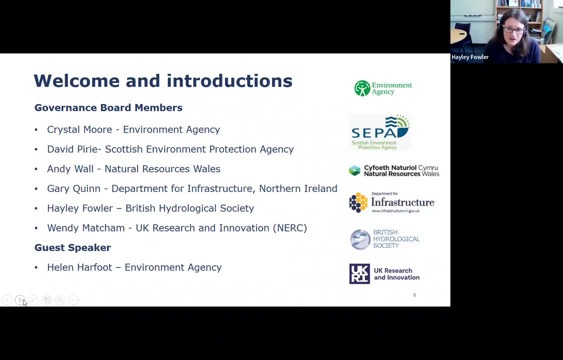 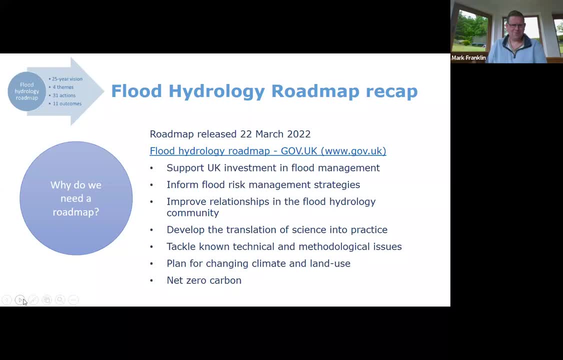 are involved in this initiative. So I'm going to move on to the next slide and hand over to Mark Brilliant. Thanks a lot, Hayley. So I'm Mark Franklin from the Scottish Environment Protection Agency. So the Flood Hydrology Roadmap is a 25-year vision. It was released in March of this. 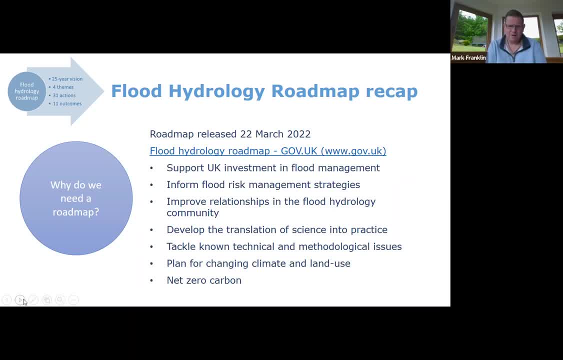 year and it's based around the realisation that I think a lot of us have had that we need to get flood hydrology right for the whole of the UK. That's getting the right investment and the right management of flooding. so to help with that, It'll be bringing in the whole flood hydrology. 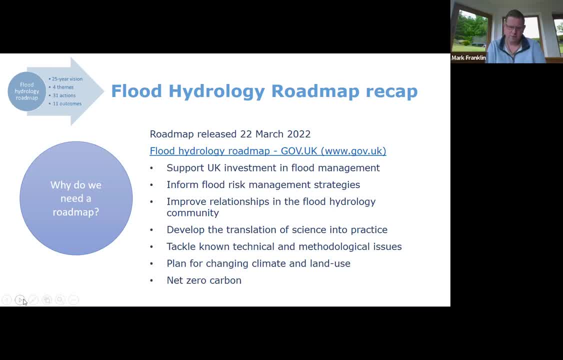 community together So that we can tackle the issues that we know about with the methods and the data, get really great research and development and get that all translated and adopted into practice so that we can actually use it to improve how we manage flooding across the whole of the United Kingdom. 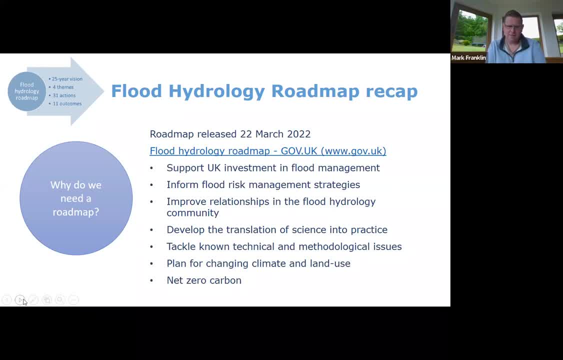 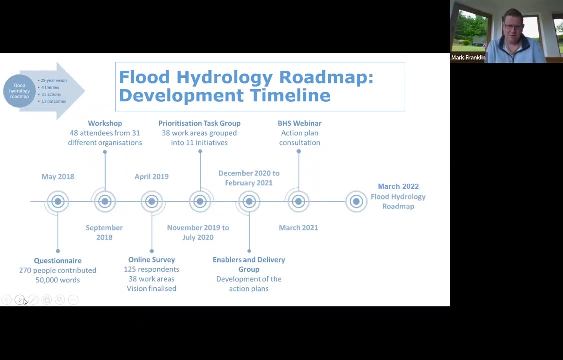 And it will be helping us plan for the changes that we're expecting with climate change and changes in land use and the transition To a net zero future as well. So next slide, please, Lucy. So we've not been doing this in isolation and we came to speak to the British Hydrological Society. 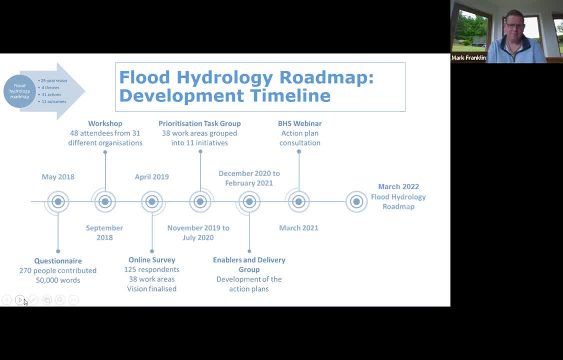 previously, but it all started back before 2018.. And in May 2018, we sent out a questionnaire which we thought about for a while, and we got really good responses back from the UK. We had a really good response from the UK flood hydrology community on there, about 270 people contributed to that. 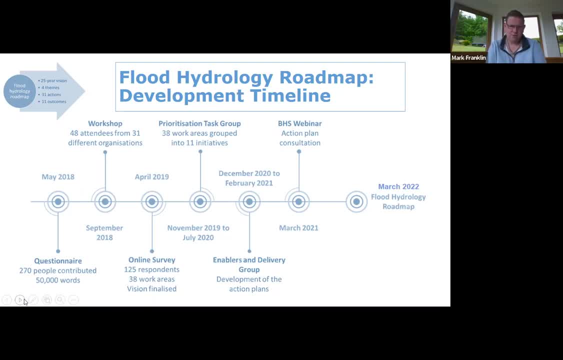 Then we took the responses from that questionnaire and held a workshop- Again really good attendance- from across a large number of different organisations across the whole of the UK and the different sectors. Again, building on that, we pulled together an online survey and again, we had a really good response to that. 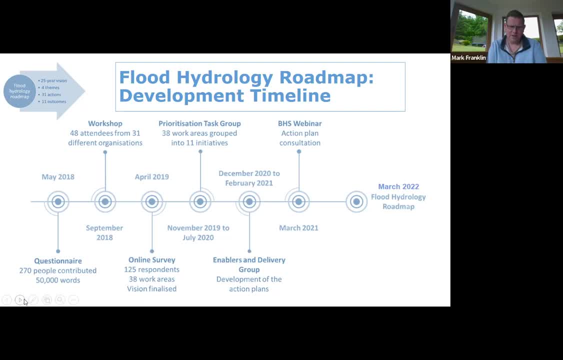 And that enabled us to get a really good response And that enabled us to start work on the vision and get that finalised. Off the back of that, we've done some work to prioritise and group all the different ideas and suggestions that we'd received from all that feedback. 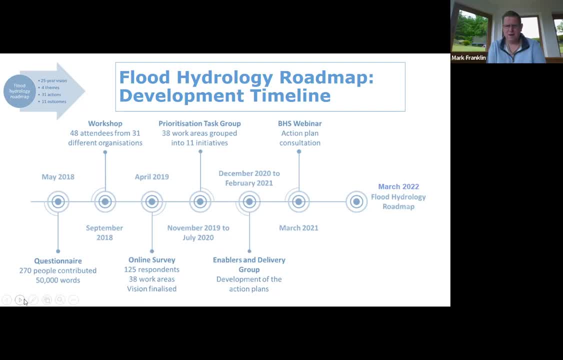 So we grouped it into around 38 different work areas and 11 initiatives, and I'll talk a bit about them. And then we've been developing action plans that enable us to deliver all the different tasks and outcomes that we need to, and they've been consulted on. 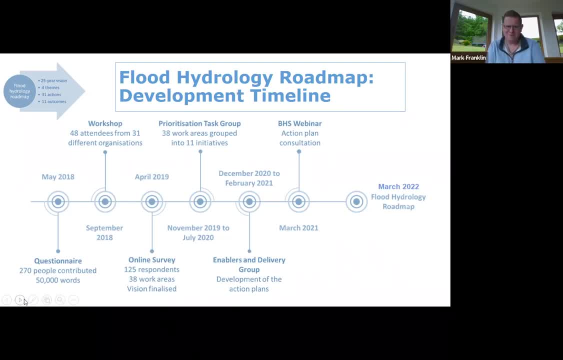 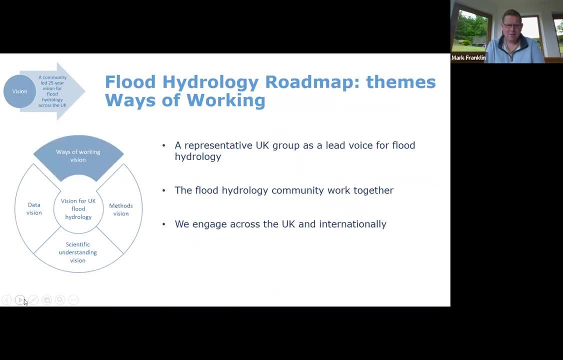 Like I say, we held the British Hydrological Society webinar back in March 21.. And then in March of this year we published the flood hydrology roadmap after that was signed off by the Governance Board, So that's available to everyone. Next slide, please, Lucy. 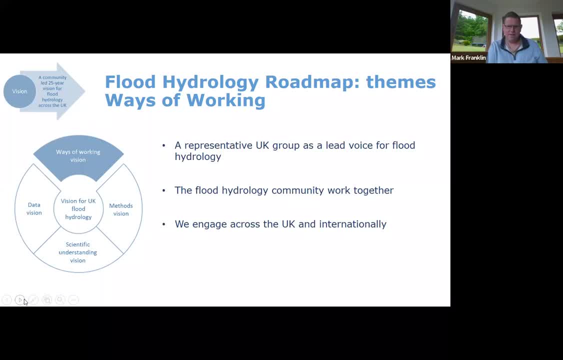 So I'm going to talk through some of the themes today. So the first thing I'm going to talk about is around the way it's working, how we want the UK flood hydrology community to work together. So we see this group and the roadmap as a lead voice for flood hydrology in the United Kingdom. 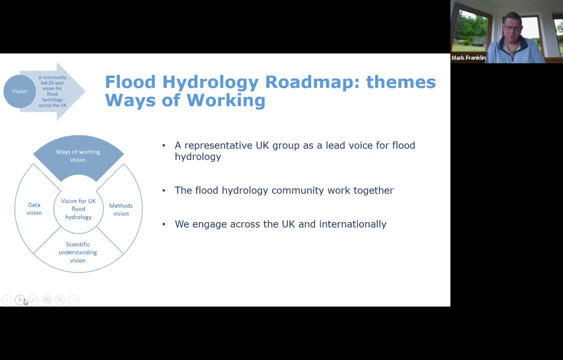 It's a unifying voice about how we can all work together in a more consistent way, how we can have really consistent and clear technical advice and guidance, and how we're going to engage both amongst the community ourselves and across internationally so that we can really 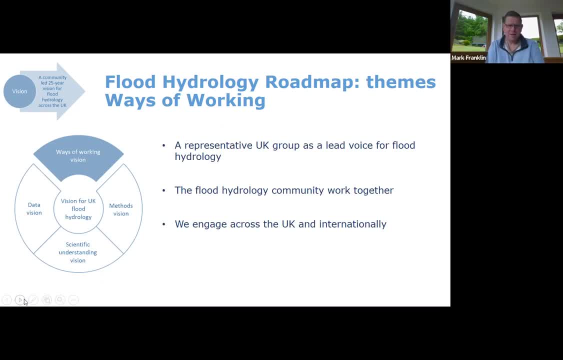 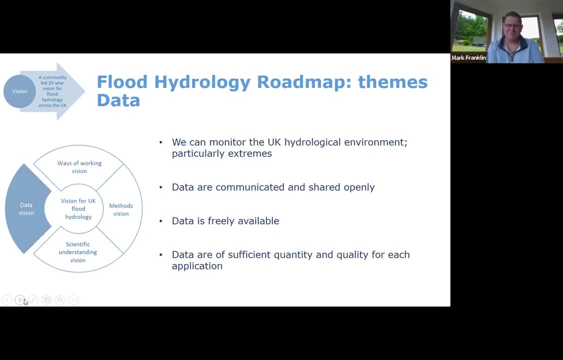 improve Efficiency and innovation. Next slide, please, Lucy. And we're also realise data is close to my heart and fundamental to everything we do, So we want to make sure that the, the network of monitoring across the whole of the UK, is funded. 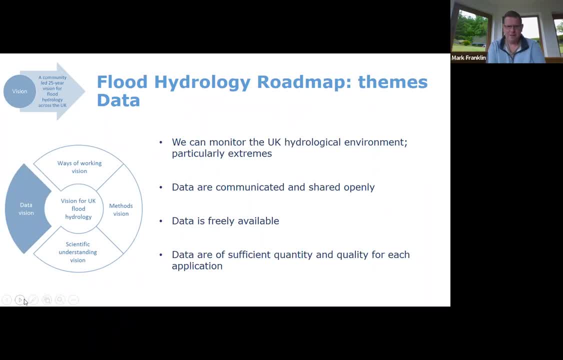 We've got the right technology skills and capacity to monitor the UK hydrological environment. We want to make sure that data is well managed, It's It's communicated, It's freely shared and freely available to everybody, and that we've got the data of the right quantity and quality for each application. 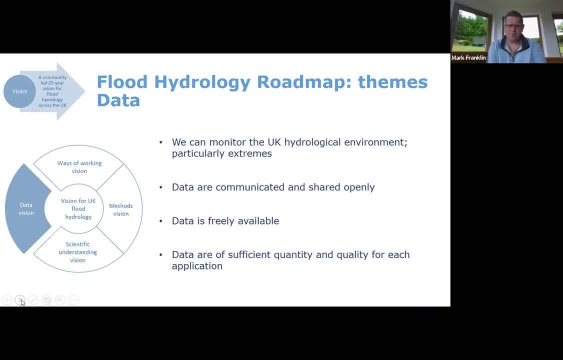 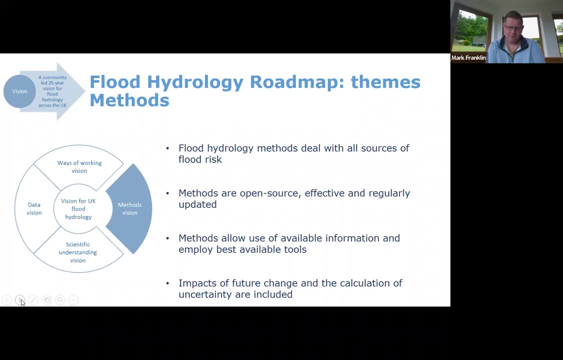 And again about having the consistency so that we know that we are collecting the right data and sharing the right data in the right ways for everybody. So next slide, please, Lucy. So the the next theme is around methods. So really importantly. 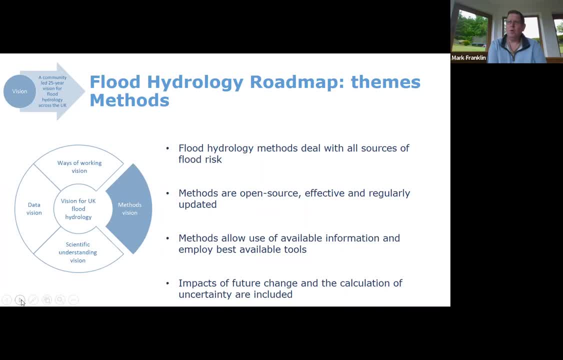 So the flood hydrology Roadmap. it considers all sources of flooding, So that's fluvial, coastal, pluvial reservoirs, considers both real time design and planning for all sources of flood risk, with driving hard to make sure that the methods and tools that are developed are open source and we want to make sure they're available and, critically, that they work well for everybody and they're supported and regularly updated. 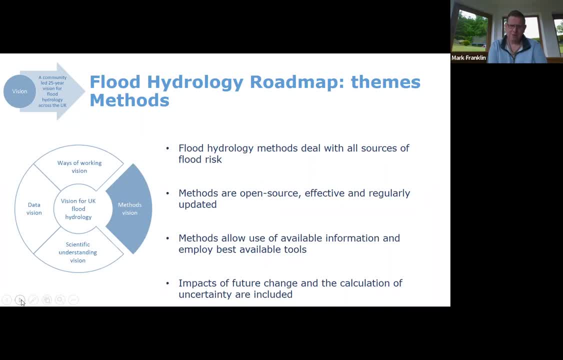 So they're. They're The best methods are available and we want to make use of the best available information. We want to be consistent, We want the data to be accessible and the methods to be accessible, and And they need to be trusted. 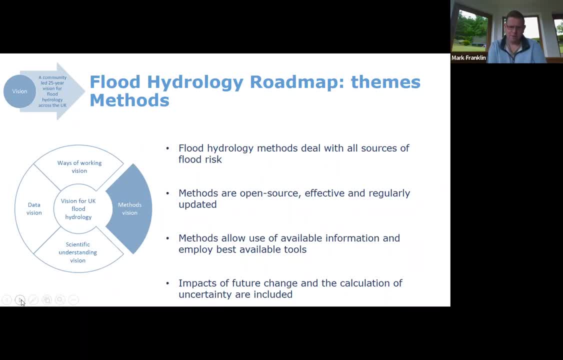 So the methods will be peer reviewed and that are used as well, And we need to consider climate change and uncertainty and make sure that we include in uncertainty in all the decisions that are made around flood risk in the UK. So we'll be driving forward to make sure that uncertainties accounted for. 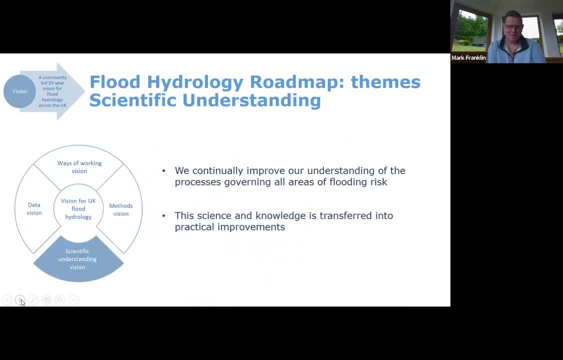 when we're doing those. So next slide, please, Lucy. So the next theme is the scientific understanding. So basically, this is about improving our understanding of all the different areas of the processes that govern flood risk And, critically, around this there's always lots. 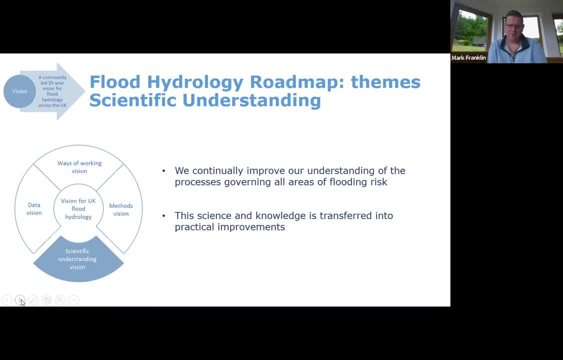 of really good science going on across the UK, But what we really want to do is make sure that that state of the art, science and technology is transferred into practical improvements. So there's a big focus on on driving all that great scientific development into something that's. 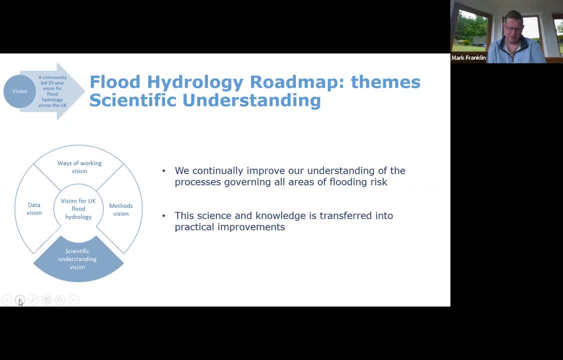 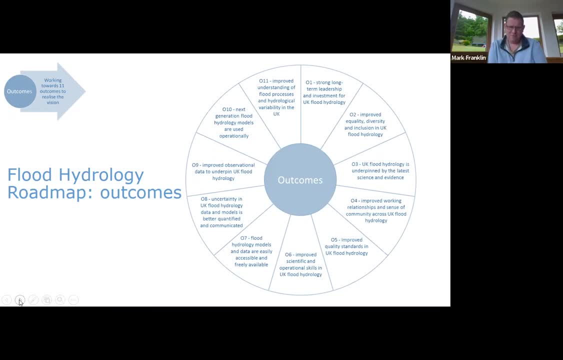 tangible and can be used practically in day to day application. Next slide: Lucy. So that's really great, laudable goals, But we need to break those down into some outcomes. So the first one is the strong leadership. So we need to break those down into some outcomes. So the first one is the 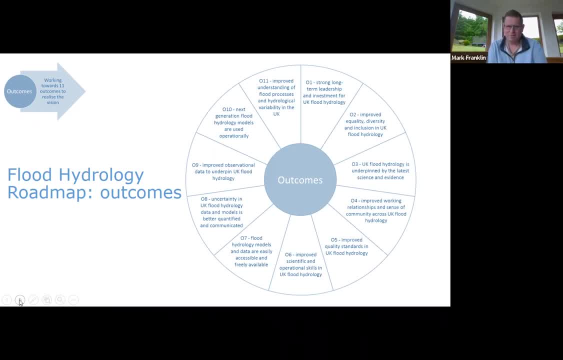 strong leadership. So we need to break those down into some outcomes. So the first one is the leadership and getting the investment in UK flood hydrology. So I'll run through these quickly. The second one is to make sure that we've got the equality, diversity and inclusion. So we're talking. 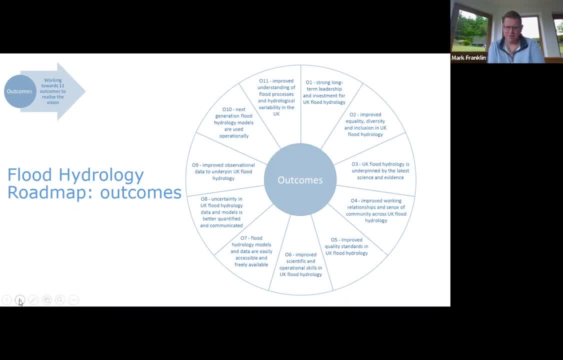 about the whole UK flood hydrology community, not just certain sectors of it, And we want to make sure that we're using and it's underpinned by the latest science and evidence. We want to improve the relationships and the community across the UK So really forming a strong flood hydrology. 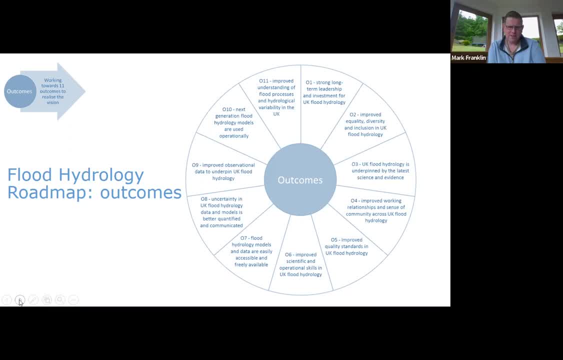 community. We want to make sure that there's quality standards and they're fit for purpose across the whole of the UK. We want to make sure there's the right skills across the whole of the UK. We want to make sure that the models and data. 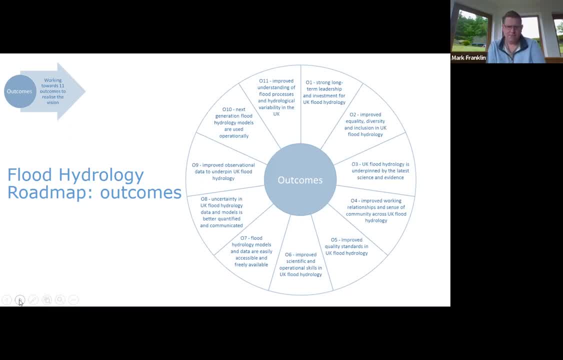 are freely accessible and freely available And we want to make sure that uncertainty is better quantified, understood in the models and the methods and better communicated. We want to make sure we've got the observational network right across the UK. We want to make sure that the next 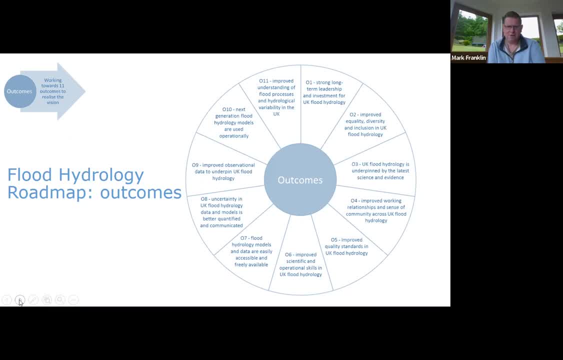 generation of flood models are being used. We want to make sure that the next generation of flood models are bought into use and are used operationally across the UK. We want to make sure that we've got an improved understanding of flood processes, hydrology and the variability of those across the. 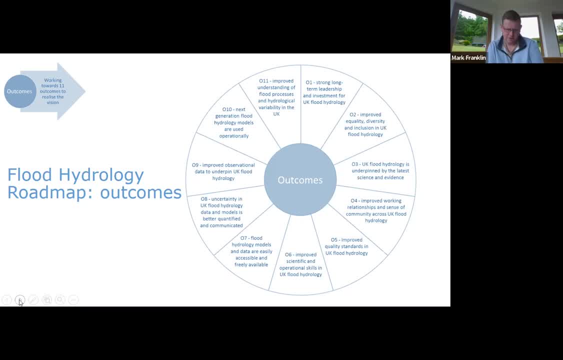 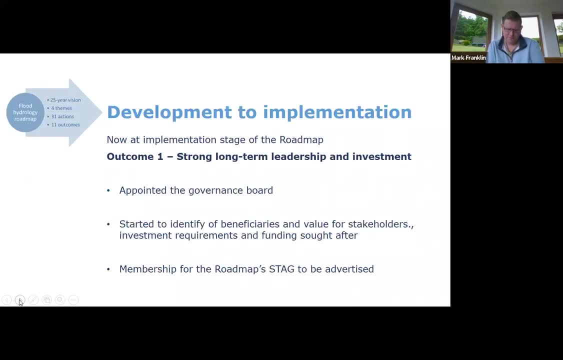 United Kingdom as well. So those are the 11 key outcomes that we're working towards. So move on, please, Lucy, to the next slide. So this is the bit now where I start talking about needing your help. So we've made a great, a great start on this. We've got the roadmap and we've made a start on 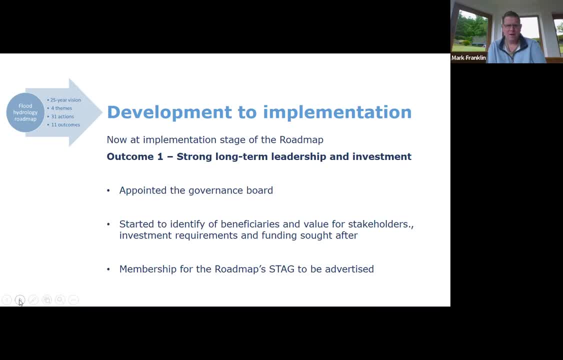 the strongly on this. We've got the roadmap and we've made a start on this. We've got the roadmap and we've made a start on the governance board- leadership and investment, So we've appointed a governance board that Hayley talked about. we've started to work out who the beneficiaries of this work are, what the value is for different stakeholders, and we're working on the funding. 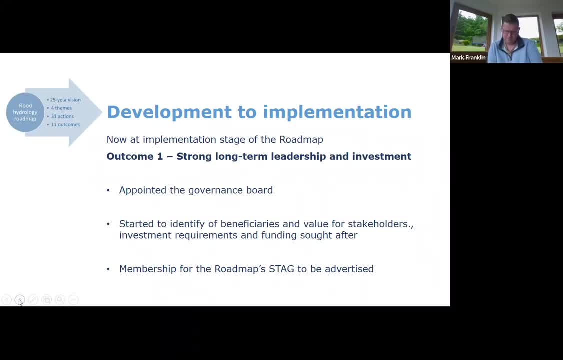 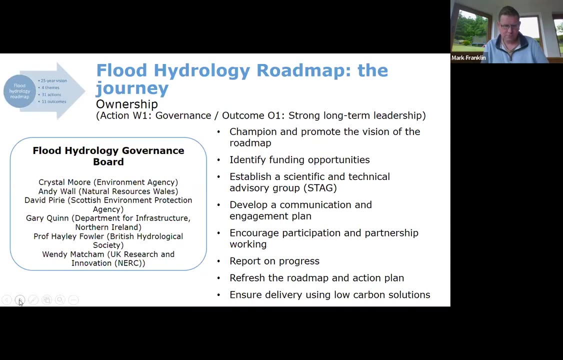 We're about to set up the Scientific and Technical Advisory Group, which makes sure we have the right scopes and outcomes for our projects, and of which the EA Flood Hydrology Improvement Programme is one of those projects. that's linked Next slide, please. So a bit more here on the governance board. 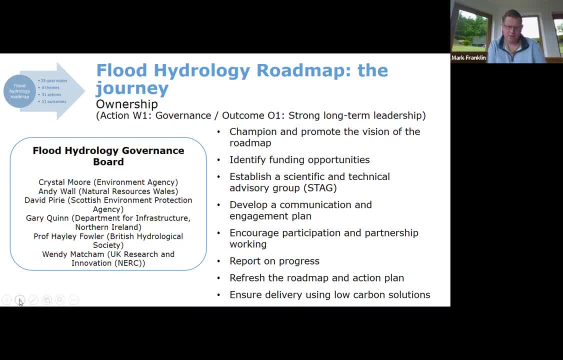 So the governance board includes potential funders from across the United Kingdom. It's here to help leverage funding, make the programme happen and help the community and the practitioners get the roadmap going. You can already. we already described who was on it, but it's a 25 year programme. 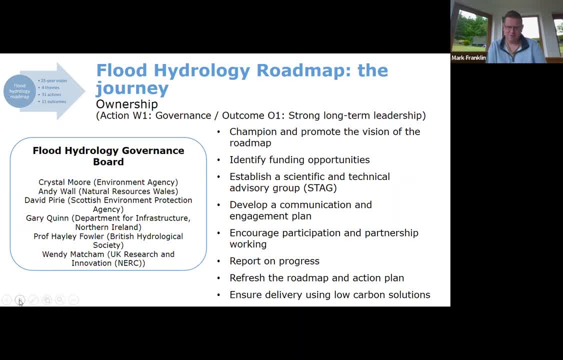 So the names will change of the people that are involved in this project through time. The scientific and technical advisory group we're setting up will lead and own technical delivery, and the governance board will be looking for funding opportunities outside government bodies to help. So from a scientific perspective, 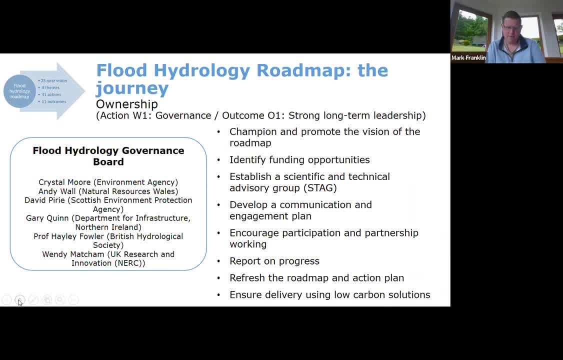 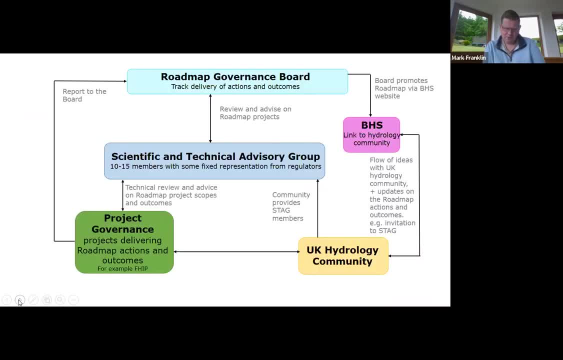 we've got an ambition to attract funding from UKRI for some of the research programmes. Next slide, please, Lucy. So just trying to show how it all fits together. So the governance board owns the roadmap programme. It tracks delivery on how things are going. 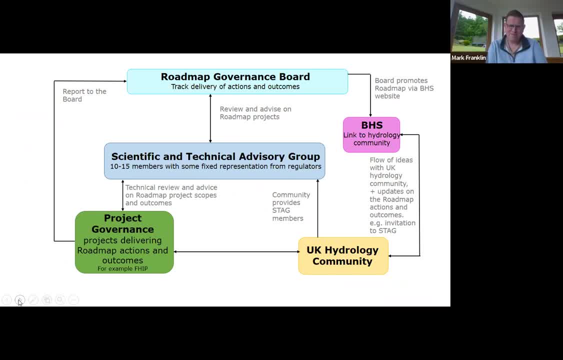 and provides leadership. We're going to work- continue to work- with the British Hydrological Society, which is our link to the community, Helps promote the roadmap, get input from the hydrological community and from different practitioners. The UK flood hydrology community will provide the members. 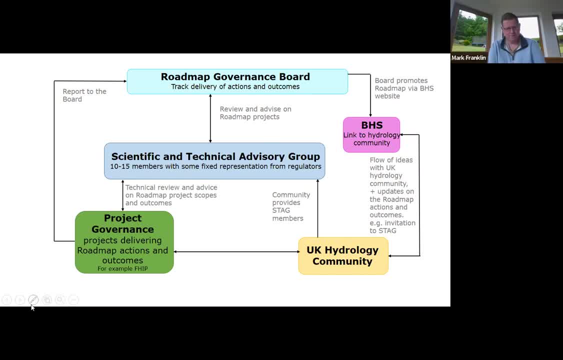 of the scientific and technical advisory group, which we're going to talk a bit about later, And the scientific and technical advisory group will be making sure that we're working on the right things and the right outcomes And, as I say, there'll be a number of different projects. 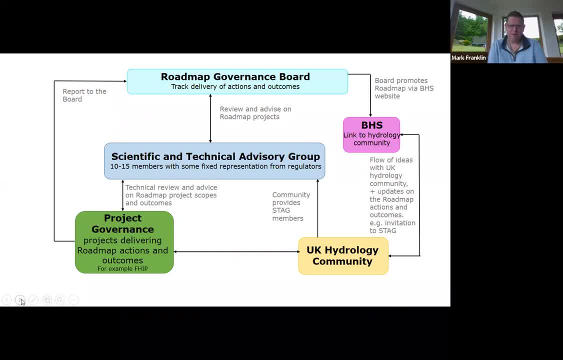 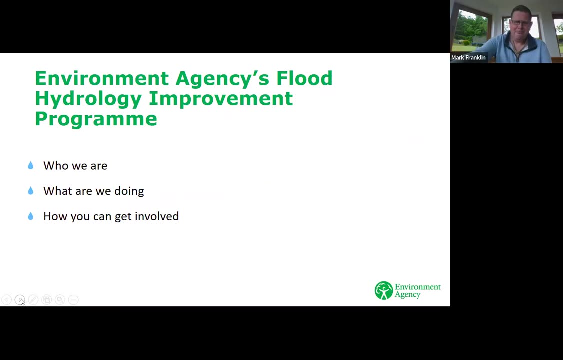 which the scientific and technical advisory group will be advising on Things like the EA flood hydrology improvements programme, which Helen's going to talk about next. So I'll hand over to Helen now, Thank you. Thanks, Mark, Afternoon everyone. 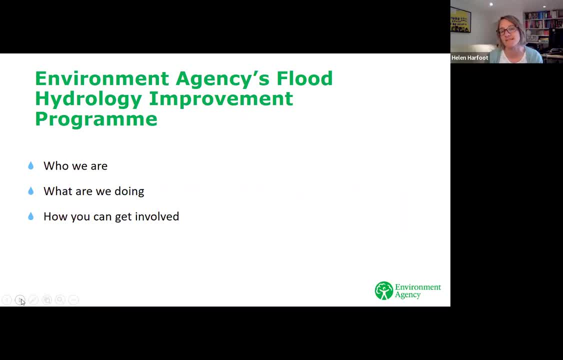 I'm Helen Harfoot and I'm the lead hydrologist for the Environment Agency's Flood Hydrology Improvements programme, And in the next few minutes I'm aiming to answer these three questions: Who we are, what we are doing and how you can get involved. 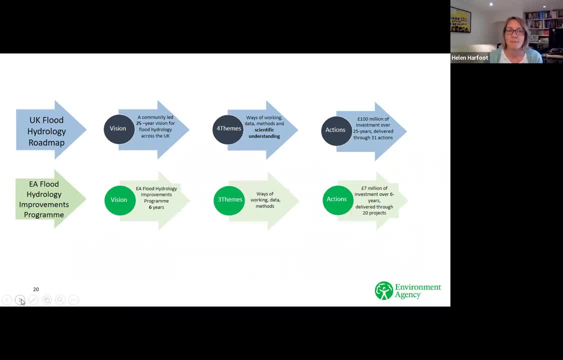 Next slide, please. So the Flood Hydrology Improvements programme program is the Environment Agency's contribution to delivery of the flood hydrology road back, and we are a seven million six-year program aiming to deliver improvements in flood hydrology both within the Environment Agency and across the wider community. and to deliver this program, the 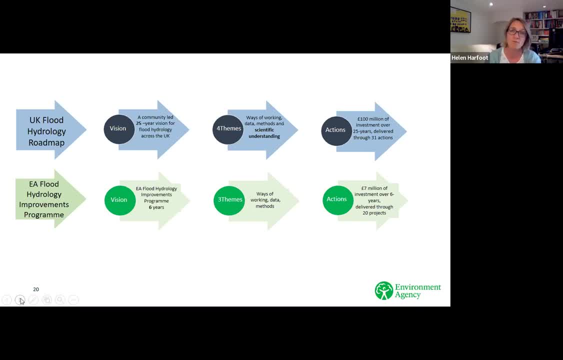 Environment Agency has created a dedicated team of project managers and hydrologists, and we've spent the past 18 months establishing a team and developing an exciting program of projects and also starting to deliver. however, the program isn't just focused on delivering project outputs. we're also interested in creating new ways of working between the Environment Agency and the 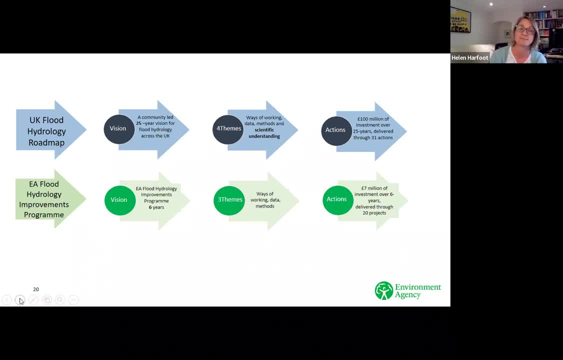 wider community and also between the UK regulators. and then linking back to the figure that Mark talked you through, the project is governed through the Environment Agency but as it seeks to implement at the end of the year, it will be implemented in the environment agency and the environment agency. 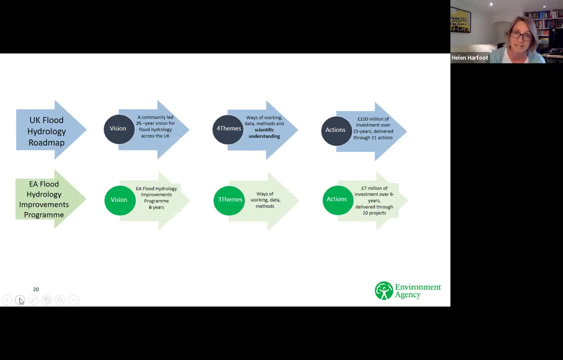 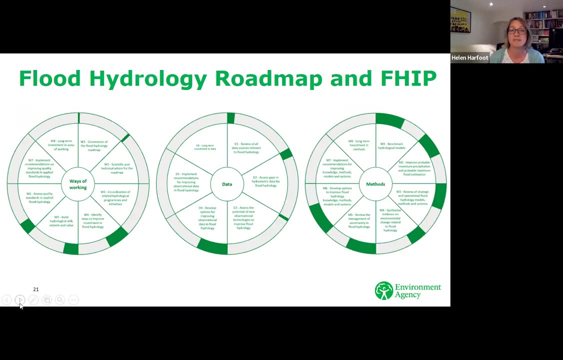 will be involved in the development of the project and we've also been working with the Environment Agency and the Environment Agency to develop a roadmap for the flood hydrology road back, and it has and will continue to see guidance and technical steer via the roadmap stag. next slide, please. for those of you familiar with the flood hydrology roadmap, you'll probably 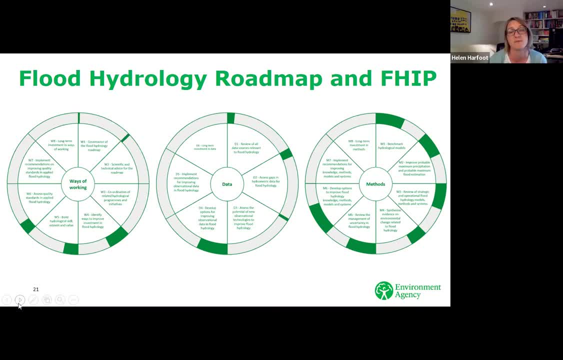 recognize these wheels as summarizing the actions for each of the three themes. we've got ways of working on the left, data in the center and methods on the right, and apologies for the small text. you can read it, but if you want to find out more about the actions, please I suggest you consult the 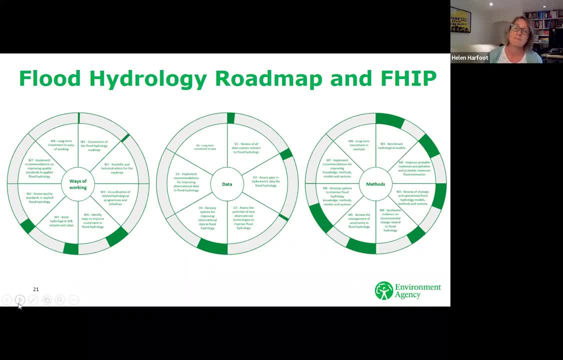 roadmap document on the dot gov website. the green shading here just indicates where we've allocated project spend against the roadmap actions, and I think the key points to note from this are that we're only looking to deliver against actions against three of the four roadmap themes. we're 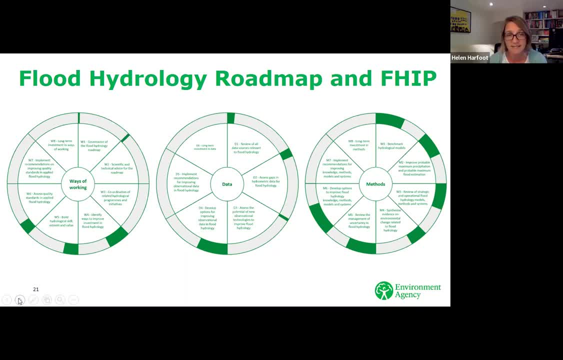 not looking to deliver any actions of within the scientific understanding theme. we're not looking to deliver any of the actions in their entirety- and this really reflects the scale of the roadmap actions- but also their complex nature and really requiring the input of more than one organization to ensure their successful delivery- and also that the majority of our funding is directed to. 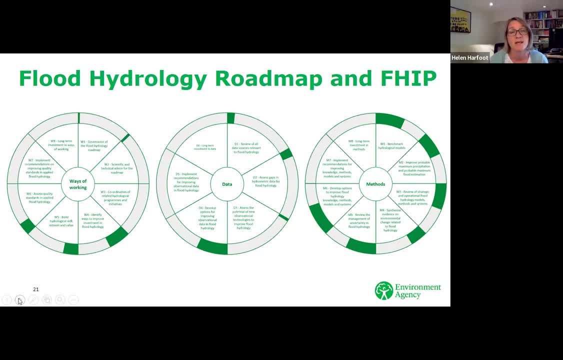 delivering actions within the methods theme of the roadmap. so we've got around 20 projects currently listed in our program and the majority of the projects especially in the ways of working and within the environment agency, but within all of the three themes and the methods theme in particular. 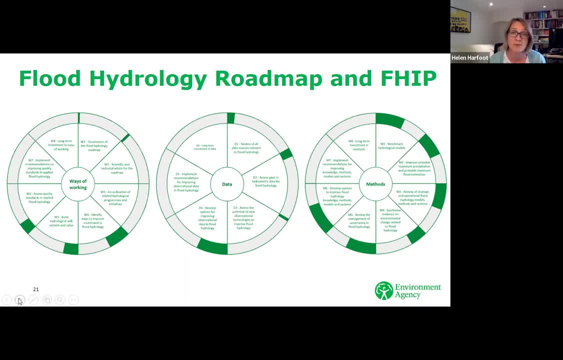 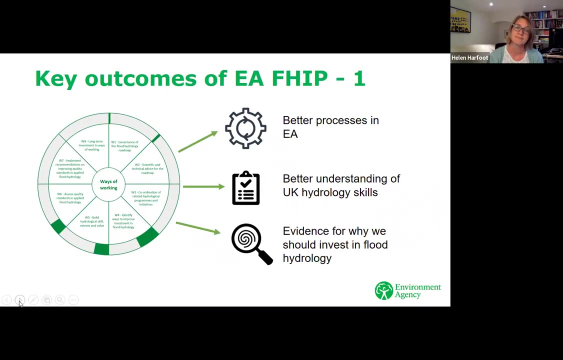 we are starting to look to address actions from the roadmap that do extend beyond England and the environment agency. so, rather than the list of the projects, I'm just going to focus on some of the key outcomes now which may be of interest to to you all. next slide, please. so within the ways of working. 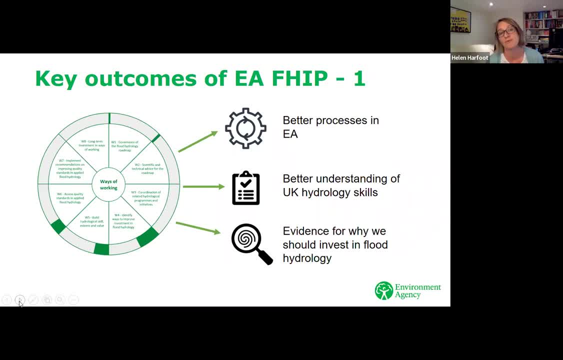 theme and we are looking to review and improve flood hydrology processes within the environment agency and as well as look at how we can better collaborate between hydrologists across the flow range within the EA. we're also planning to work with BHS regulators across the UK, industry and academia to learn more about the experience skills diversity. 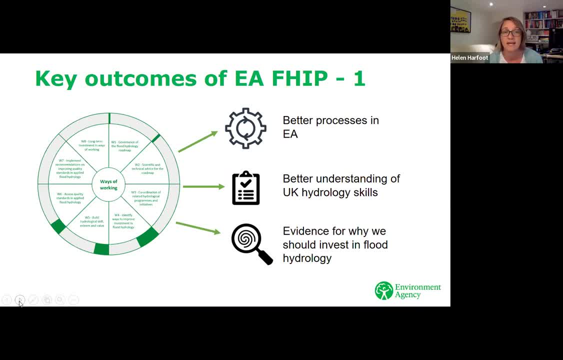 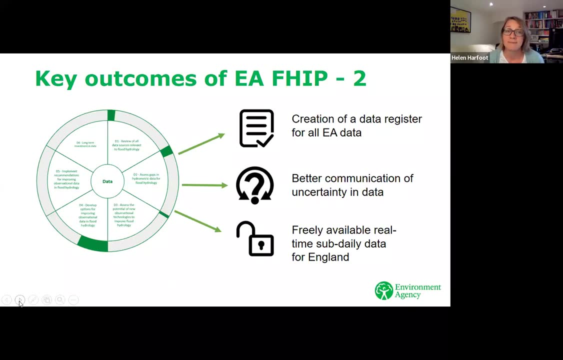 and satisfaction of hydrologists practicing in the UK, and this will be via a skill survey, and then we're also looking to gather evidence on why we need to invest in improvements in flood hydrology. next slide, please. within the data theme, we'll be looking to scope and develop a data. 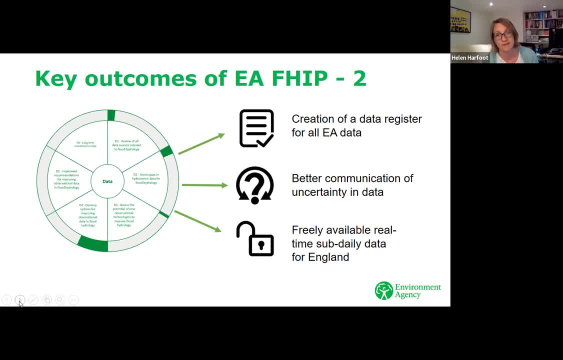 register, which will be accessible via the dot gov website, and the intention is that this would deliver a go-to source for knowing what data we hold, how to access it and, hopefully, to improve understanding on issues relating to the data. the quality of the data we're also looking to review. 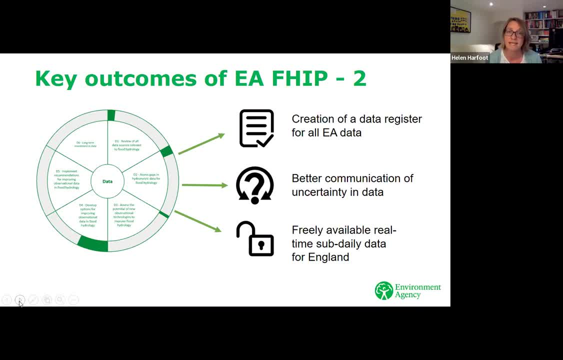 how we quantify uncertainty and hydrometric data within the environment agency and how we might improve how we communicate this to users of our data. and we're also planning on making our sub-daily data freely available in real time to download by the environment agency API, and this will be for the full period of record for all. 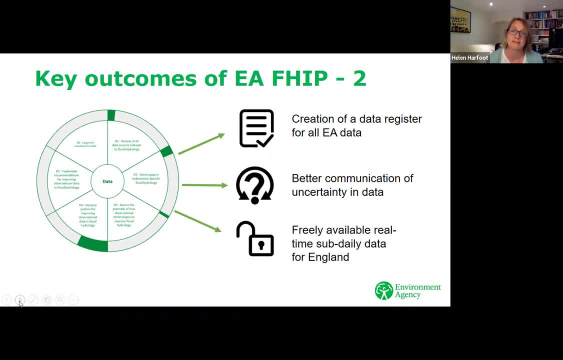 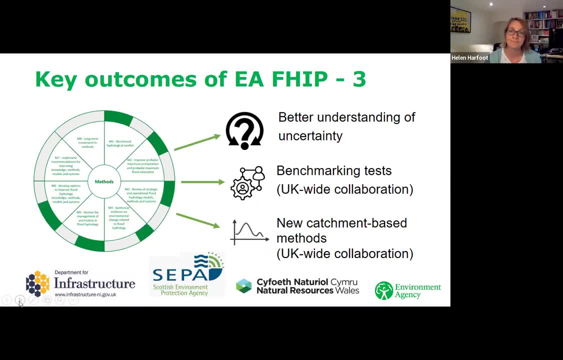 our active flow level, groundwater and rainfall data sites that are currently held on our whiskey archive. next slide, please. within the methods theme, we've just finished the project which looked at relative uncertainties in the modeling chain and we're planning to use the outputs of this project along with future projects. 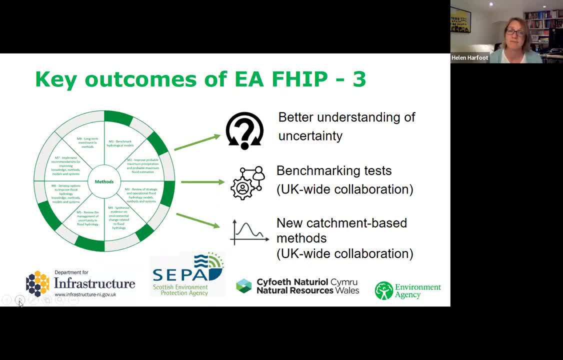 to better communicate the uncertainty that we all know is inherent in flood estimation, and this will be to benefit our decision makers. and then, for the last two outcomes that are listed here, we're looking to work with colleagues from SEPA, NRW and DFI to develop new ways of working to create 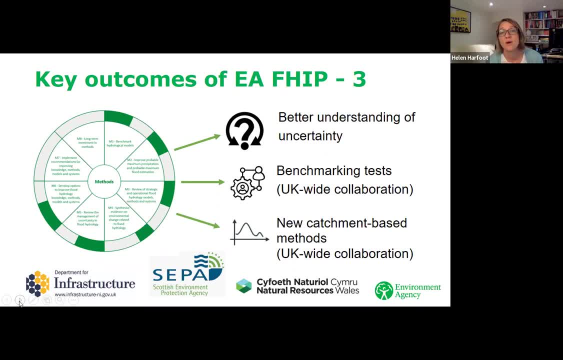 outcomes for benefit across the UK. so this includes benchmarking tests for hydrological models, and the scope of this will be co-developed in due course, but we're expecting it to include evaluation criteria of both model performance alongside how it meets user needs. and then, secondly, we're planning to consider 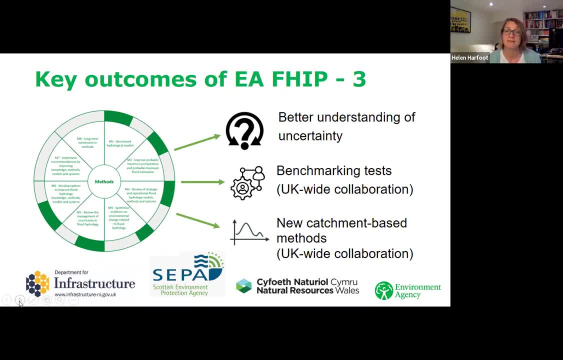 the introduction of new to operation catchment based methods that could serve as an alternative and not a replacement for current methods. we do not anticipate that the program will have the opportunity to actually embed these new methods, but will provide an opportunity, a proof of concept, which will hopefully highlight the benefits that 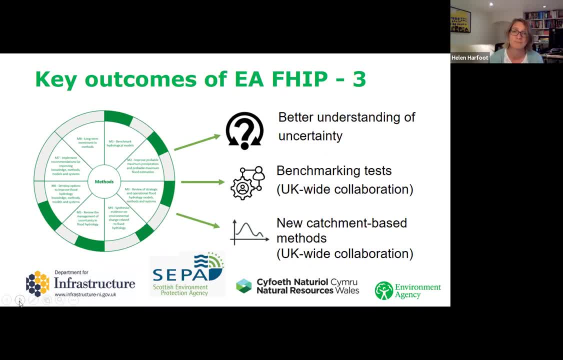 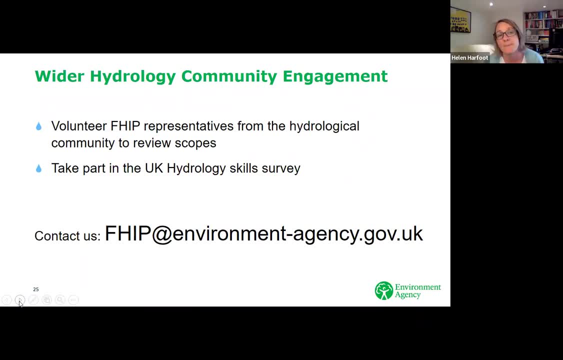 such methods could bring to operational flood hydrology. next slide, please. and finally, how can you get involved- and I hope that many of you on the call today were involved in the creation of the flood hydrology roadmap. we are really keen to continue to external voices in the delivery of our program, so one way we're seeking to achieve this is through 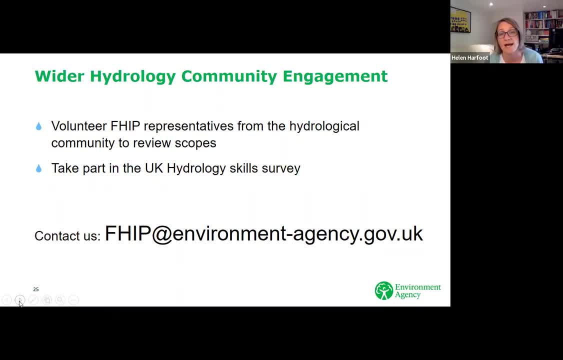 the creation of a community rep role, and these are people who can review our draft scopes and deliverables and provide us with feedback, and I'd like to say a huge thank you to those of you who have volunteered for this role so far. we've been really grateful for the feedback that we've 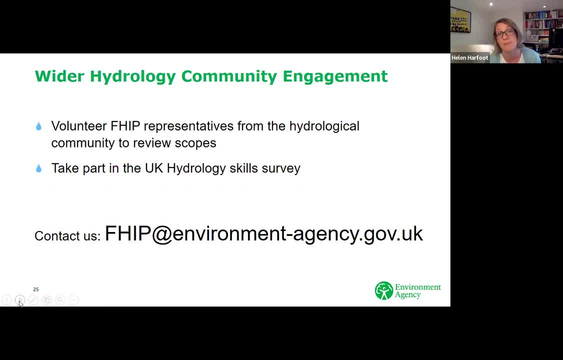 received. so if you are interested in being a community rep on a future fit project, please look out for calls to apply via the BHS mailing list and also via our web page, which we hope to be on the BHS website within well, within the next few weeks. and please also keep an eye out for our UK. 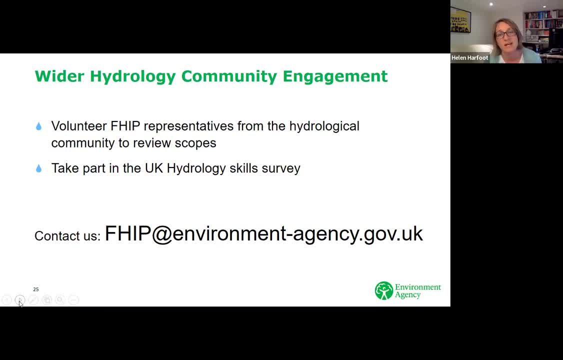 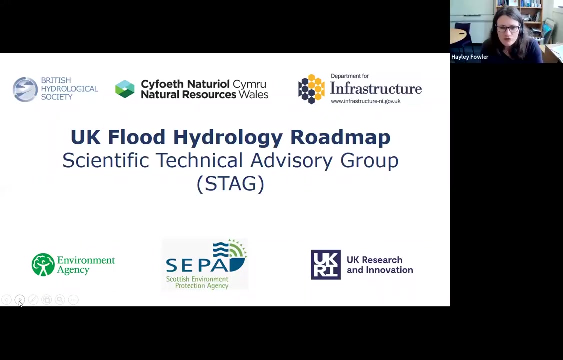 wide skill survey and, more importantly, take part. we're really keen to hear more about you and our hydrology community. and then, finally, another option. another option or another way to get involved is via the roadmap stag, which Hayley will talk you through now. thanks, Helen. right, so the the stag is another way that you can get involved in supporting. 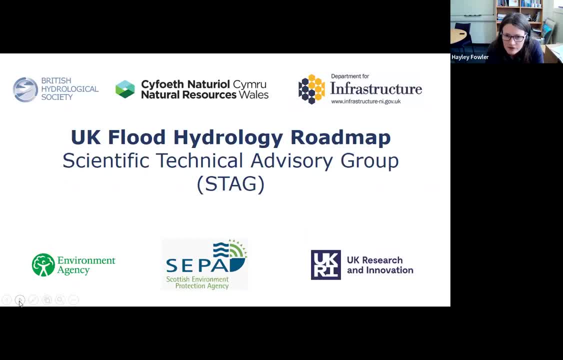 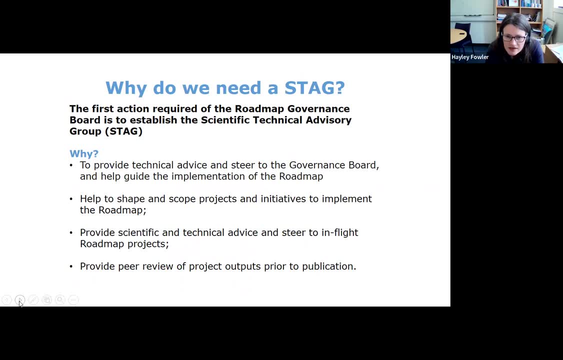 and more closely supporting, I suppose the UK flood hydrology roadmap next slide Lucy. so we we need a stag, basically Boättcher will the base- I think it says Britain and a straightforwardCan Iarme. thank you, civil. This is Steven Goodman. one effectiveness support project, honoured economic frame Stage where profit andài. 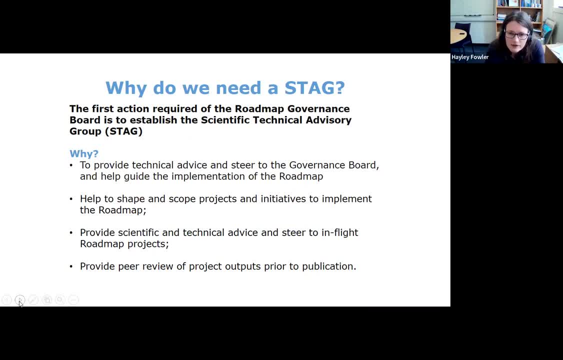 management of business analysis. cancel us all the scum together to provide technical advice and study the governance board and to help guide the implementation to road map dsブуль- not apply co swap and scope projects and scientific and technical advice and peer review of project outputs prior to publication in one of the first actions required of the governance board was to actually establish this scientific technical advisory group, our Un caveat. 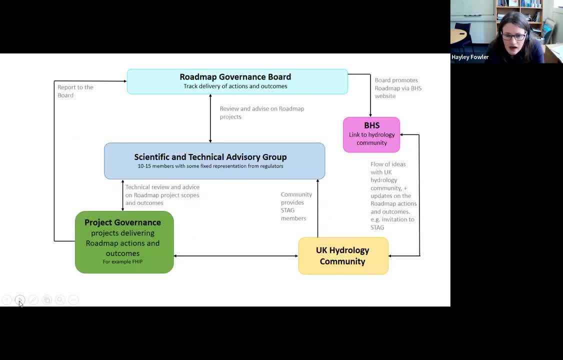 Yes, what writing pei already. Mark showed this slide as well, and the scientific and technical advisory group were very much seeing this as a group of around 10 to 15 people with- as I'll give a bit more detail in a second- some fixed representation from from the regulators working very closely with the roadmap. 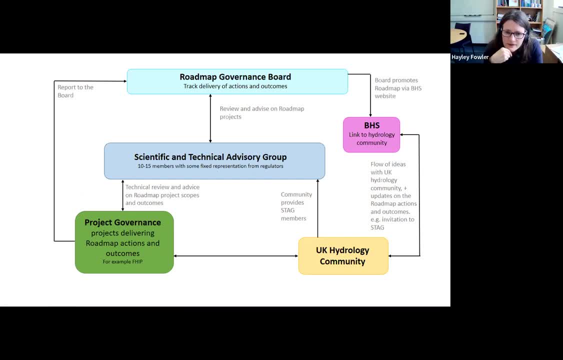 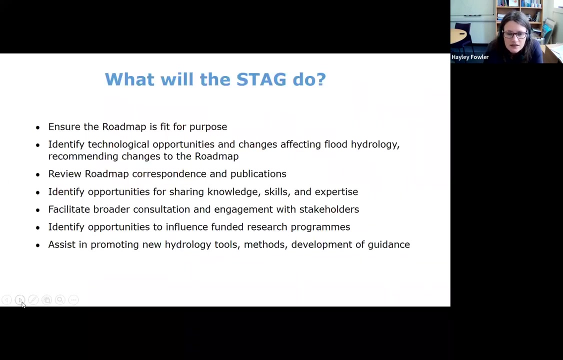 governance board in terms of reviewing and advising on the roadmap projects in terms of scientific and technical capacity, but also providing links to the UK hydrological community and to provide links to the project governance as well. so next slide, Lucy. so I mean, I've basically said a lot of these already, but I think really, we're, you know, we're- 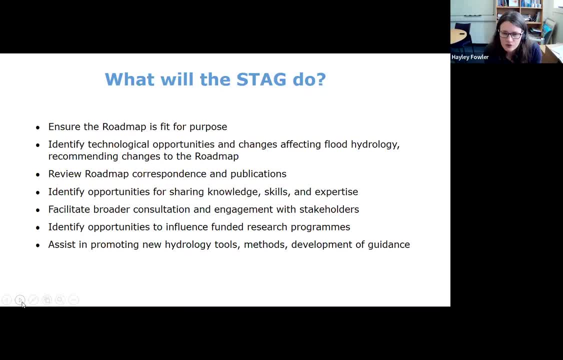 looking for people to provide this scientific and technical support um to the governance board around the priorities in the roadmap um, and particularly um thinking about um opportunities to influence funded research um which can be taken up by the governance board um to assist with the promotion of of new tools, methods and development of guidance. 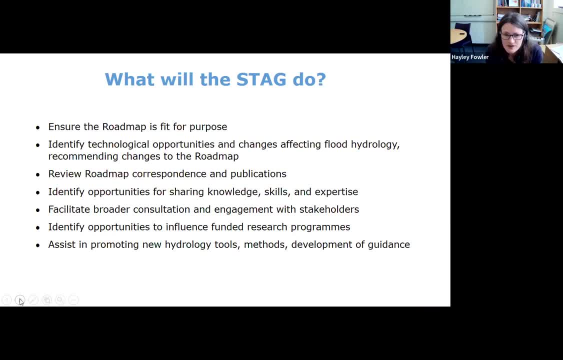 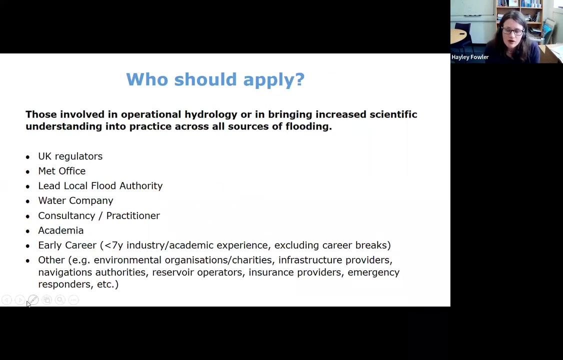 to facilitate this broader engagement with stakeholders um to to, obviously, um look at uh supporting projects and identifying um and reviewing uh projects after they happen as well. um next slide, lucy. so, um, we've got a list of people here, really, who we envisage being part of. 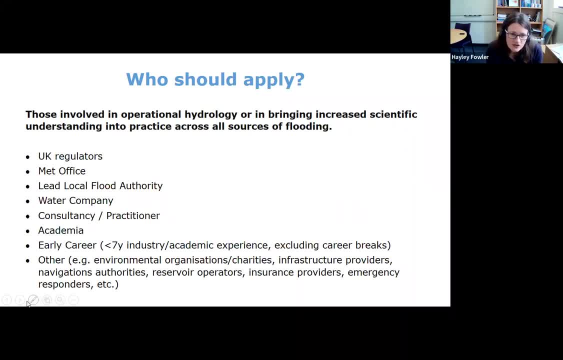 the um, stag, um, and in particular, just to stress that um basically we're looking for for anyone involved in operational hydrology or bringing increased scientific understanding to the practice across all sources of flooding. so we're looking for a wide range of expertise here, um, and we're not just looking for established um. you know the usual suspects, although very 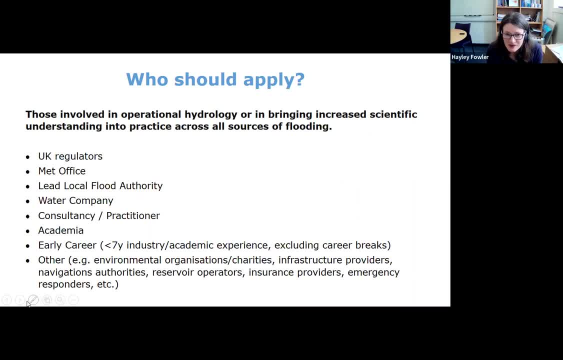 welcome as well, but we're also looking for for early career people and people who haven't been involved in this type of thing before. um, so again, we're going to have representation from the uk regulators, from the met office, uh, the lead local flood authorities, the water water companies, uh. 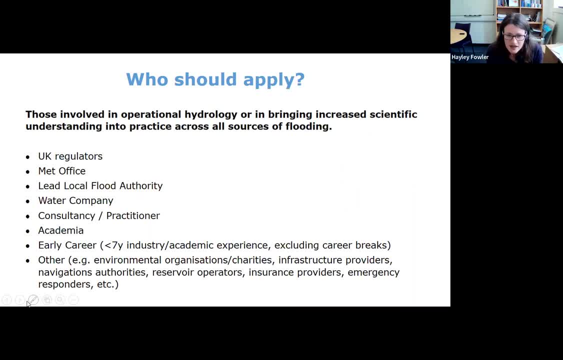 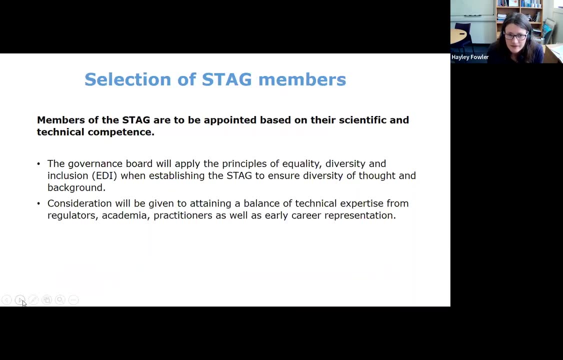 consultancy, practitioners, academia, early career, as i say, and others um, for example, organized environmental organizations and charities, infrastructure providers, for example, reservoir operators, insurance, emergency responders, etc. next slide, lucy um. we will have an application process um and the governance board will decide on the um, the membership of the stag um and that's going to. 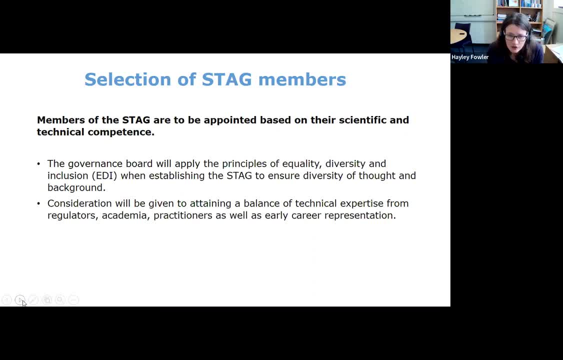 be basically um appointed based on scientific and technical competence. um. we're looking to apply, obviously, the principles of uh equality, diversity and inclusion, very much so when establishing the stag, and and that's very much to ensure diversity of thought and background um as well as, for example, career experience etc. um as well as the sort of scientific, technical competence across. 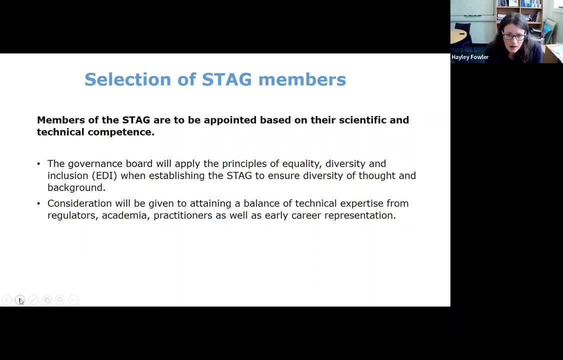 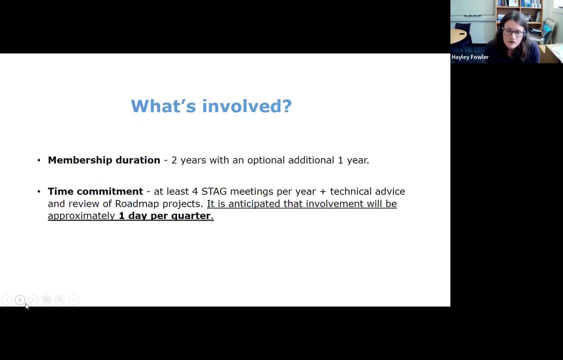 the areas that are needed um lucy next slide um. so we've envisaged a membership duration of two years initially, with an optional additional one year um and the time commitment required will be um. there'll be at least four stag meetings per year. now, at the moment, the governance board meets six times a year. 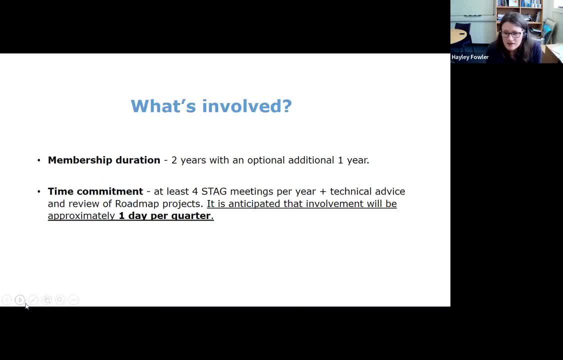 um so there'll be four stag meetings and um also the need to provide technical advice and review of roadmap projects as well. um so we'll be looking forward to that. um so we'll be looking forward to as as as needed. um so at the moment, it's anticipated the involvement will be about: 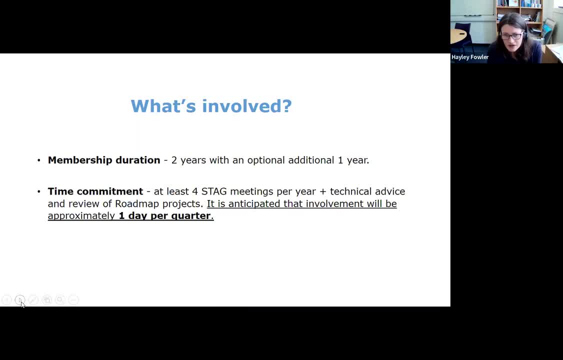 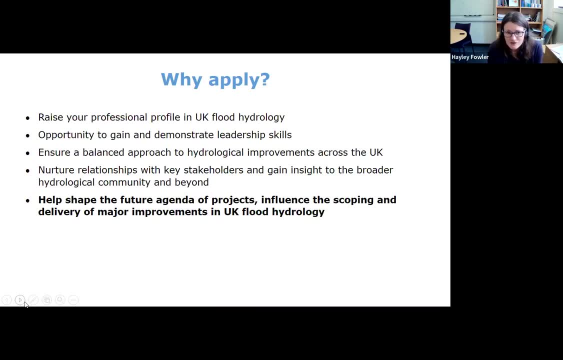 one day per quarter. next slide, lucy. so i mean, i think there's lots of reasons to apply. i think it's a really exciting initiative. it's going to be, um, you know, the the, the way we we want to do flood hydrology in the future, and it's that path for the next 25 years. so why not get involved? it'll. 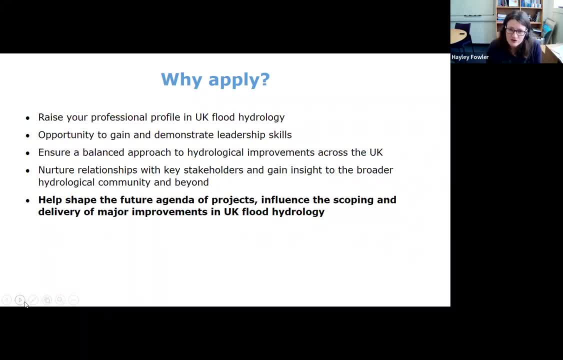 help to raise your professional profile in uk flood hydrology. um, you'll get to uh gain and demonstrate leadership skills. um, i think that getting that diversity of people involved in the stag is really important to ensure a balanced approach to hydrological improvements across the uk. um, you also get to to obviously network, um to nurture relationships with key stakeholders and 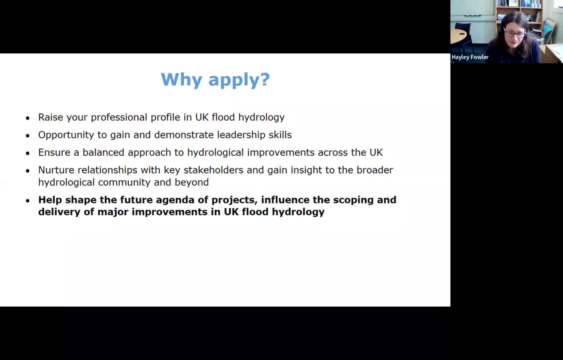 gain insight to the broader hydrological community and beyond and, most importantly i suppose you get to know the people involved in the stag and get to know the people involved in the hydrological community and get to help shape the future agenda of the projects in the roadmap um and the scoping. 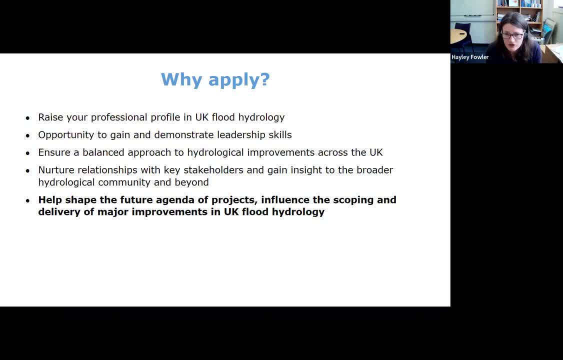 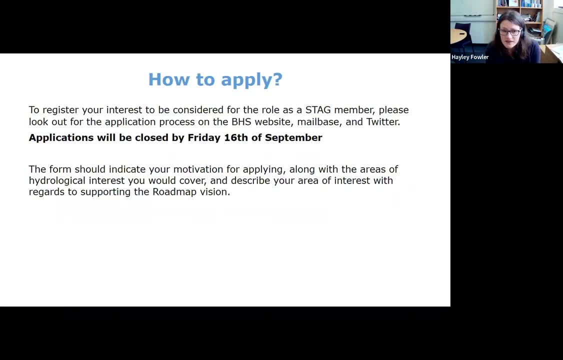 and delivery of major improvements in uk flood hydrology. uh lucy, next slide um, so um. if you would like to be considered um as a member of the stag, then, um, we're going to have a website going um, a web page, i suppose, going live on the british hydrological society website. now that will happen. 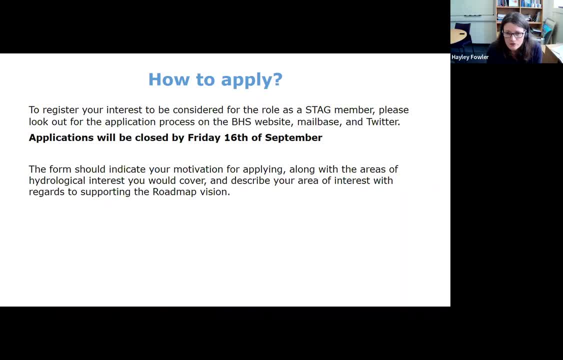 uh, by the end of this week, um, so that will detail the process for actually applying, um, and we'll also detail some more information about the flood hydrology roadmap itself, um, but we'll also put out um something on the mail base, um, and on twitter as well, um, and applications will be closed by 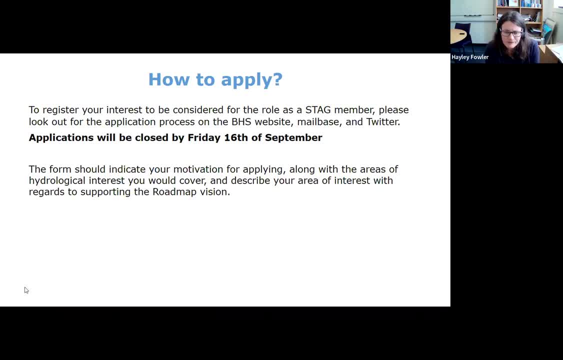 friday, the 16th of september. so we'll have. we're basically doing this via an online form, which the link, as i say, will be in the description of this video. so if you're interested in doing this, it will be on this, uh, on the website and mail base, etc. um, and the form should indicate your. 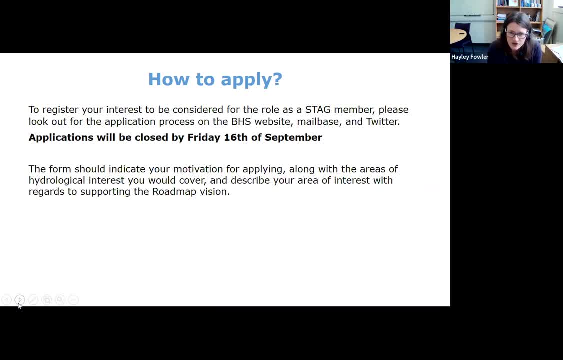 motivation for applying, along with the areas of hydrological interest, you would cover um, and also why you know why you'd like to be uh, be uh, considered um, and how you can support the roadmap vision as well. what, what technical and scientific expertise you have. so so any. 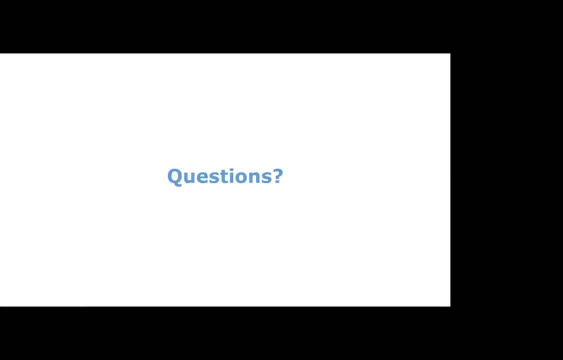 questions from anybody. hi, lucy, how are you? michael here? um, i was just wondering: is there currently a list of the projects that, uh, have been funded, will be funded? um, maybe i've just missed that, but i'm interested in so maybe. i mean, maybe either helen or mark could say something about that. but 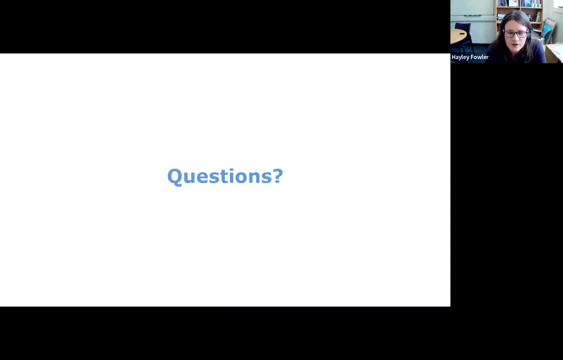 um, i think it was on one of helen's slides- um, some of the funding that's been allocated by the environment agency already for the flood hydrology improvement project, and i think it's the improvements program. um, very much so. you'd like to say something? 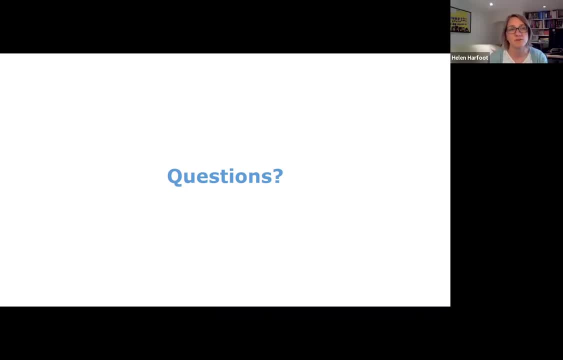 about that, helen? yeah, i well, i just wondered if the question was more broadly about projects funded under the roadmap or specifically the improvements program. um, the improvements program initially, but um, um, yeah, also interested in other. so obviously we have, we have a list of projects and we're just looking at how we 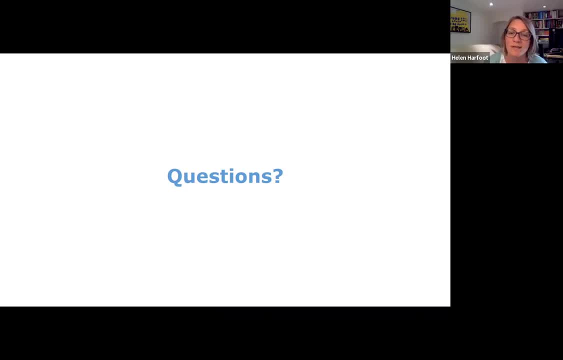 can best share um, the, the growth nonsense, but also the, the fragmentation, the, the uh, the, the the start side of um. the project is doing a lot of work on the sort ofقول, the obstruction goal of the state, the for of Powder, to get that complete work going. 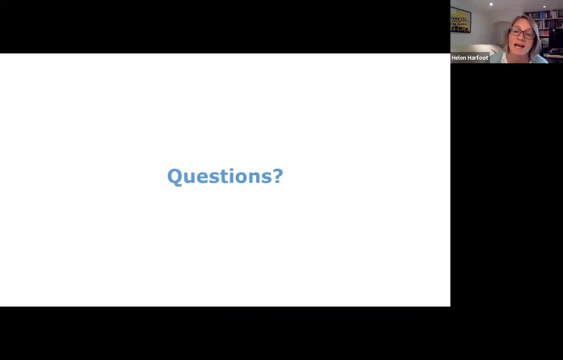 เอر tempsем our projects and our outputs, and we're hoping to have a web page that we'll be able to access via the VHS website, but this is still in construction, so if you want to have a list in the meantime, please email us, Lucy, because I don't know whether you can easily skip back. 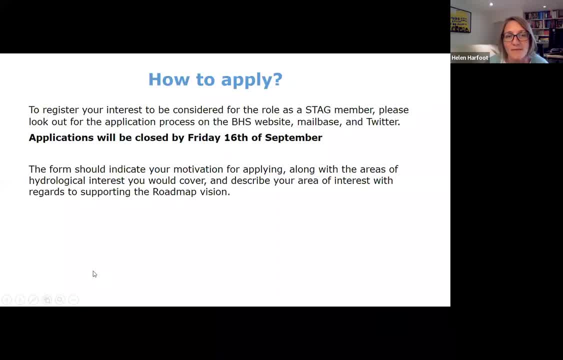 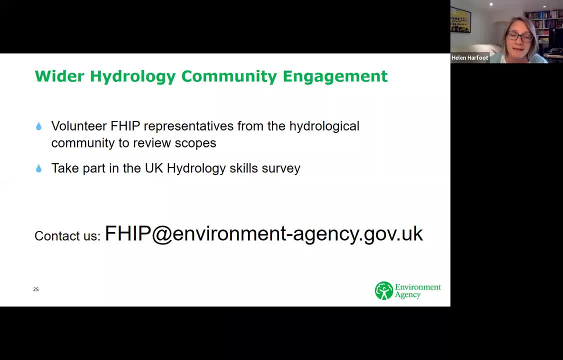 but I did put our web address at the end of my presentation, so please email us and we can send you further details on them, but we will be making, and we've got plans to make that more widely available in the coming months. Thanks, Helen. We've got some more questions coming through, so 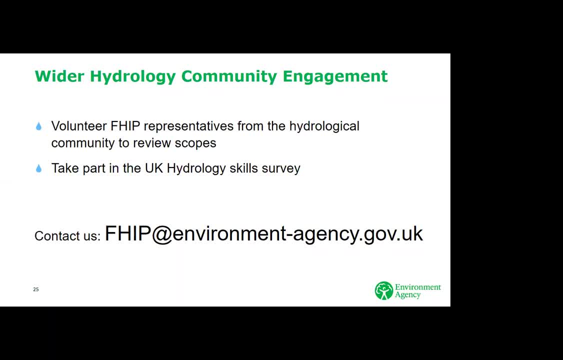 Paul, I don't know if you want to ask your question in person. Paul and Linda, Hi, can you hear me? Yes, we can hear you. Sorry, I'm doing this on the mobile and it's a little dodgy. It was maybe a daft question, but if you had a massively granular rainfall, 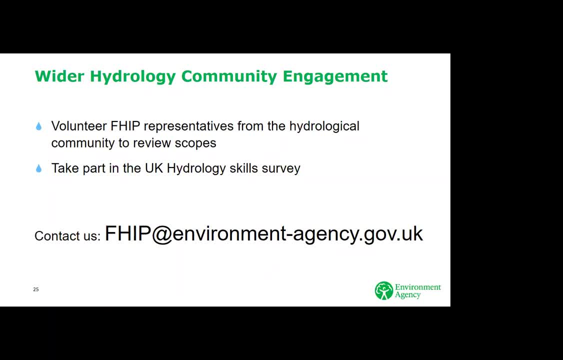 gauge network, thinking Scotland-wide, multiple thousands. would that be of use? That's possibly the daft question. The thing is, it's a future aspiration, but who best to start with? I'm going to speak to now about data formats and standards, so that we design it properly. 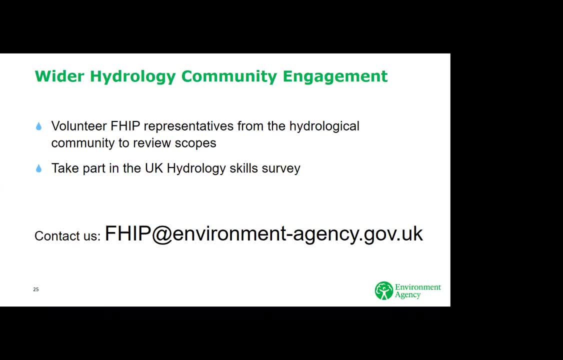 We're going to deliver it, but we want it to be of maximum use. Yeah, I mean, absolutely would be of huge value. I mean, the more data we have, I think the more. the more we can understand about processes, you know, the better we can make forecasts and all. 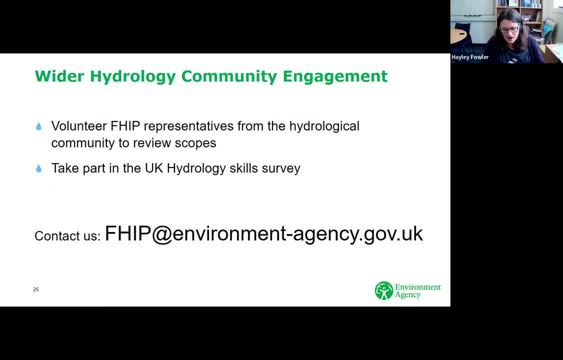 sorts of things. So it's really of great value, And I think this comes in under the data strand of the flood hydrology roadmap. very much so about thinking about new data sources, Data standards. I'm not sure exactly which part that comes under. Maybe Mark can say something about more. more about that. 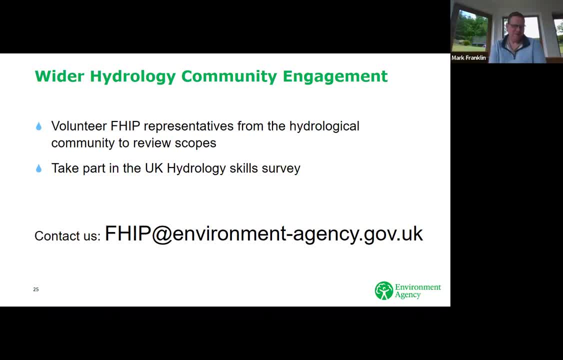 Yeah, I think it's in the data bit higher, Paul. So I think Scotland-specific Paul, you come talk to me, that'll be good. But more widely, yeah, so in the flood hydrology roadmap we're looking at where the main sources of flood risk are across the UK and all this is the plan anyway. and then 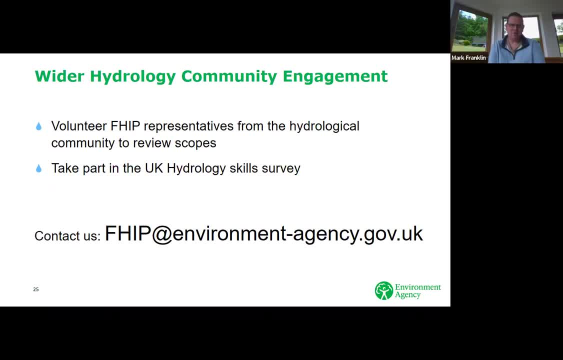 looking at what monitoring networks we need in order to support those in the future for all the needs that we've got, and then, as part of that, the monitoring network, of course, is broader than just sticking kit out into the field. So that's about how we bring the data in, what standards that's. in how it's kind of archived and shared. Yeah, I think that's a really good point. I think it's a really good point. I think it's a really good. So that's about how we bring the data in what standards. that's in how it's kind of archived and shared, and. 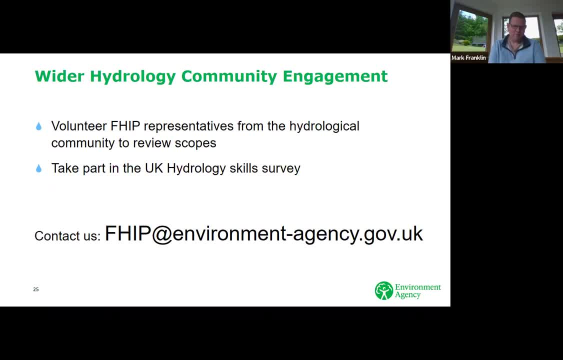 made, And then I think it's also important to really understand where the standard is and what it's freely available. so, again, a kind of theme that runs through all of this stuff is making sure we're targeting um the development on the right areas of work for the future flood risk and we're 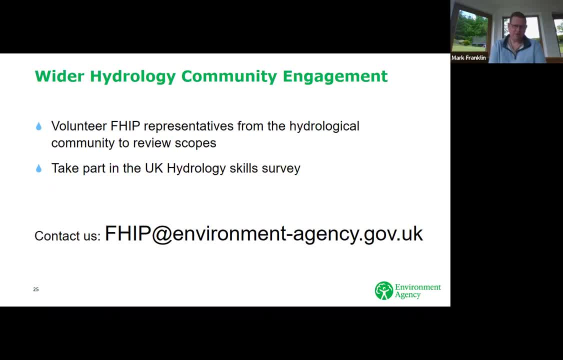 making sure that the method and the data and the technology is is transferable and easy for open access and easy to share into the right standard. so hopefully that helps, paul, thank you, you. thanks, mark um, we have a question from duncan faulkner which possibly leaves on quite nicely. 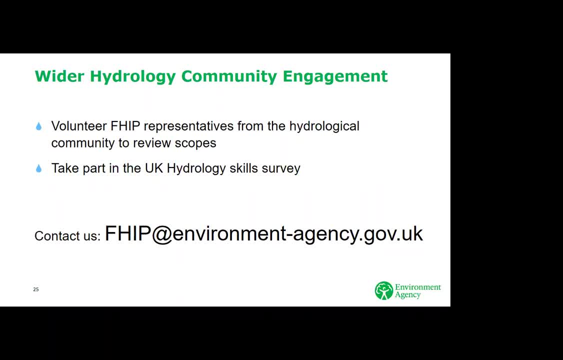 from that this point which, and duncan asks: would anyone from cpa, nrw or dfi like to comment on any plans they might have to carry out a program complementary to the ea's um flood hydrology improvement program? that's probably me to carry on going, isn't it? 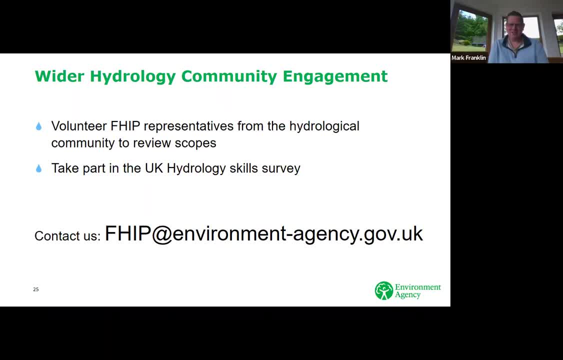 on behalf of all the devolved administrations. uh, so the plan is the. so the ea flood hydrology improvements program was already in in flight, if you like, duncan, so that's kind of ahead of the other organizations. that the plan with this whole? uh, flood hydrology roadmap. 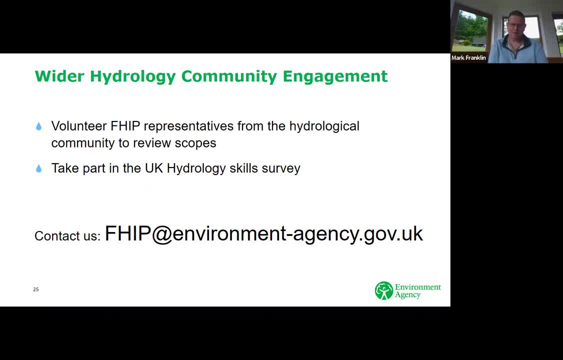 is where it makes sense, we do it together and we do it kind of once for the ea. so, um, that program is what we're we're working up now. so we started working on, out of all the different activities that are going on, what where the interest is kind of across uk where the 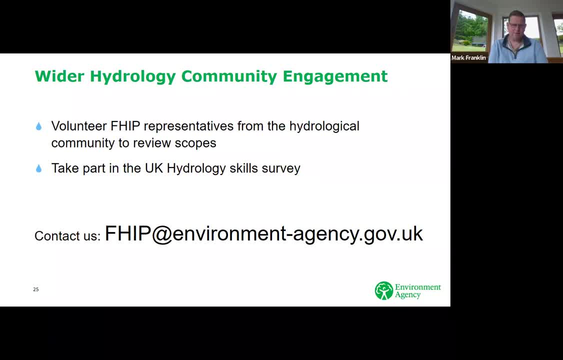 interest is um only in certain parts of the the different organizations, because we've all got slightly different uh remits and flooding uh issues, so that's been being worked up now. so the idea is, though, that we'll come together and push that forward jointly where it makes sense. 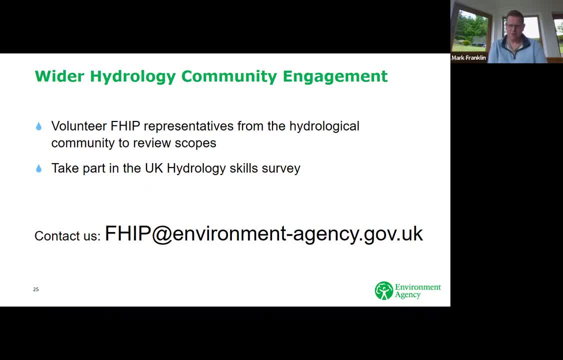 and we'll expand the scopes of some of the later flood hydrology improvements program that the ea is running to include other parts of the geography of the uk where that makes um sense also. so that's that's coming and that's definitely the vision in the 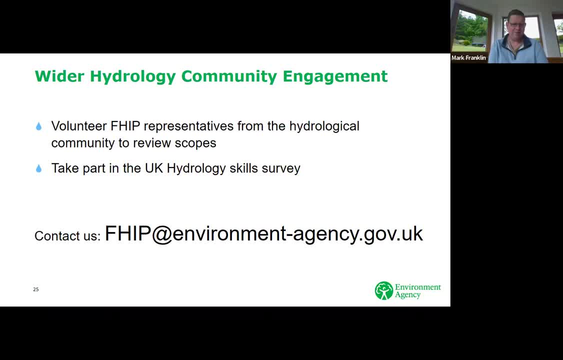 next couple of years that we're doing that um a lot better than we are now. great thanks, mark um. we have a coming back to michael's question on the list of projects as part of fhip. uh, rosswoods asks: have any of the projects in the ea's fhip already produced reports and, if yes, are they available? 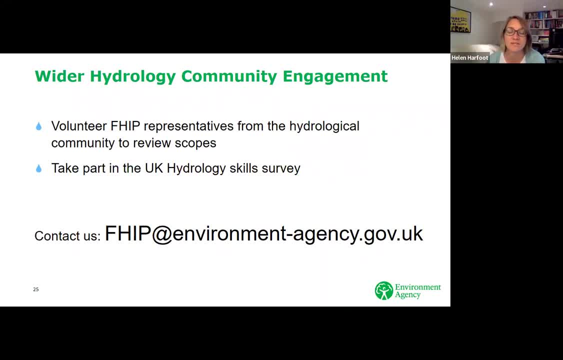 um, hi ross. um, we haven't yet got any reports that are finalized to share, but, uh, when we do, we will be um sharing them through our web page on the bhs website when we have that set up. but i said earlier that we we haven't quite set that up, so you haven't missed anything yet. 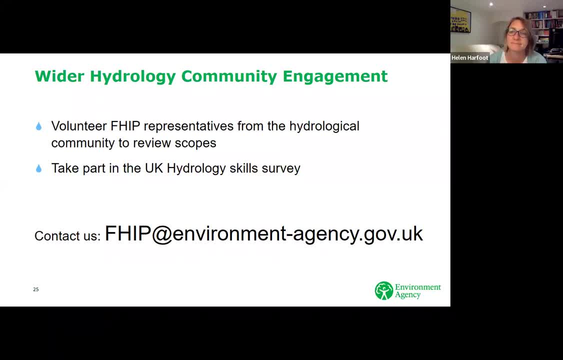 um. so we had a question um about whether the road map includes um urban flash flooding from um acid? um. if somebody would like to take that one, any of us can. yes, it covers all sources of of fhip um. so we've got a question here um. 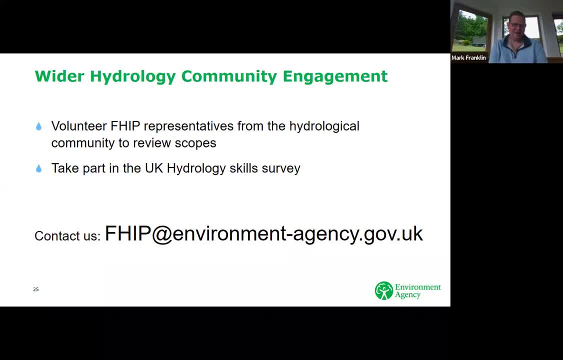 about whether the road map includes um urban flash flooding from um acid. if somebody would like to take that one, any of us can. yes, it covers all sources of of fhip. um, so we've got a question here. um, so urban flash flooding is in there. in terms of understanding that, how we 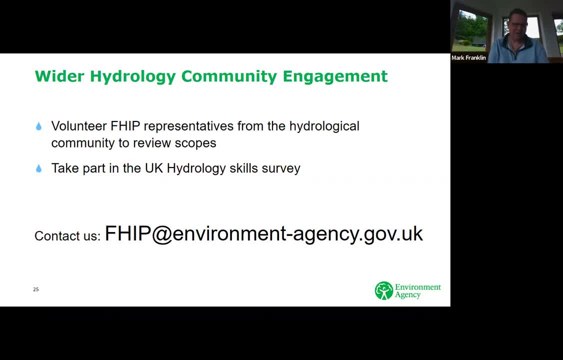 model that, what information we need to to be able to understand that and work out how we best manage um and respond to that risk. great thanks, mark um. uh, claire waller has asked a question that i was going to ask um and she says: how will the roadmap team work with nurk to join up funding for scientific 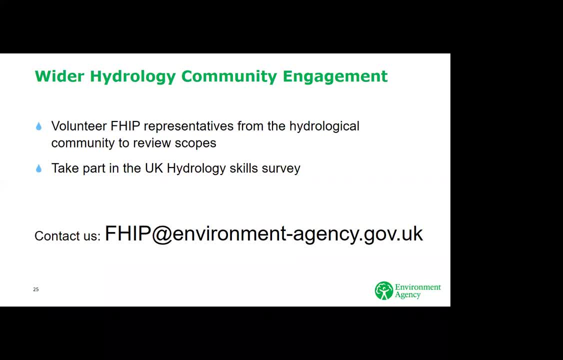 research which isn't, which isn't going to be the same as the road map team, work with nurk to join up funding for scientific research which isn't being progressed through the fhip um, and i was thinking in particular about um, the fdri program that's just been um announced, so i don't know who would like to um comment on that. 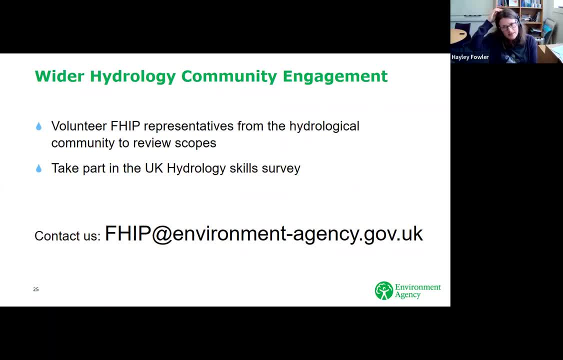 well, i mean, there's a, there's a comment in the chat and it is a standing item for the governance board um funding, um, we very much want to uh set up the stag, the scientific and technical advisory group, um as well. um, but you know, you've, you've seen that ukri are actually stat sitting on the 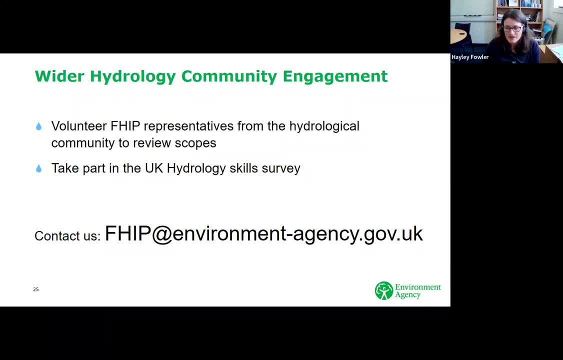 the governance board. so they have a very, very central role in this um and part of the job of the governance board is to actually identify um. i suppose you know the priorities and for funding um and part of the, the job of the the stag, is to advise the governance board. 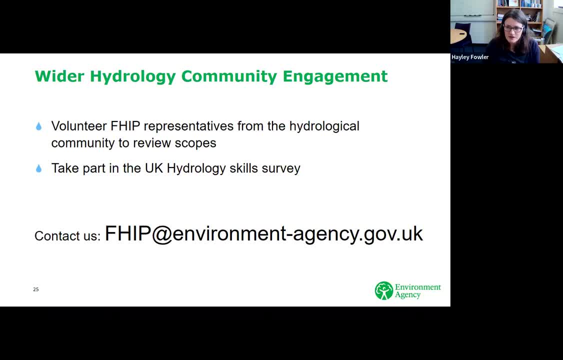 on those priorities as well, when it's formed in terms of the, the actual road map itself, um and then um. you know, we join up with nurk to basically identify um programs that they can, they can fund to actually deliver those priorities. so i think that's how it's going to work. um and yeah. 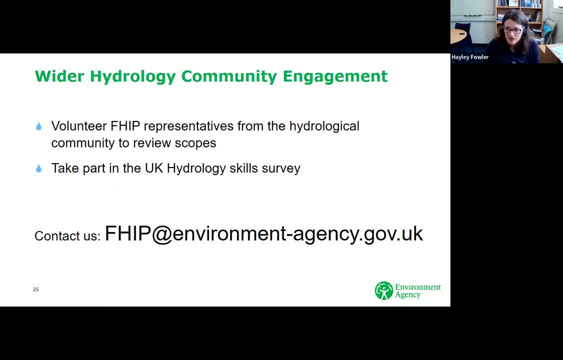 obviously there's. there's a massive investment already through the fdri project. that very much links to the road map. great thanks, hayley. and then steve cole's just popped the um link to a note about fdri in the chat. if anyone wants to add anything to that um, i think that's a great point. 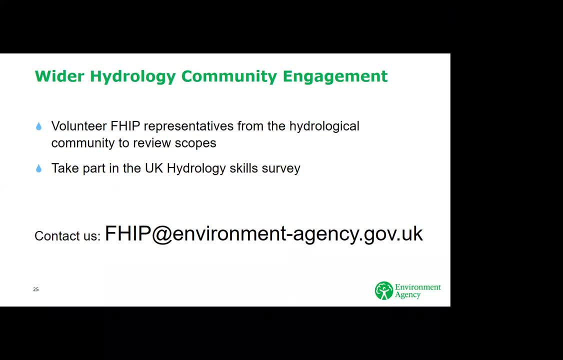 anyone wants to find out more about that? um, do we have any more uh questions from anyone? i can't. i think i've addressed all of the. come back to all of the ones already. um, yes, another one's just popped up. um, will the ea look to incorporate the outcomes of the? 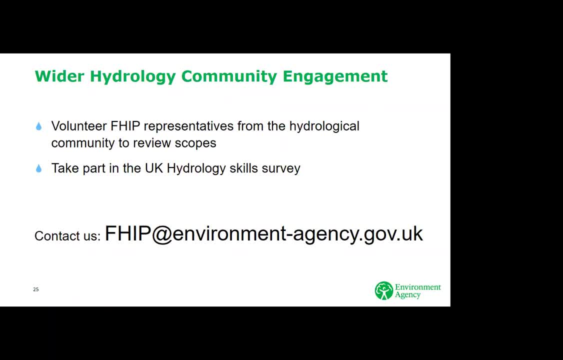 uncertainty in the modeling chain project into revised ea flood estimation guidelines and or fluvial modeling standards. thank you, andrew question. hi andrew, um, that's a really good question, the um, i don't think we'll be planning to put the the outcomes of this immediate piece. 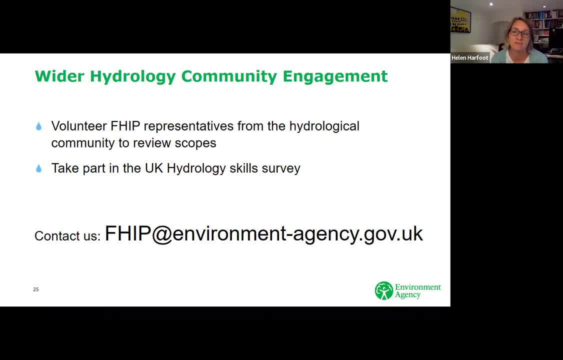 of work, because i don't think that it. it translates neatly into the to the guidelines which are due to be updated. but, um, i think there is intention that that uncertainty will be something that we need to to think about more in the guidelines in due course. so i 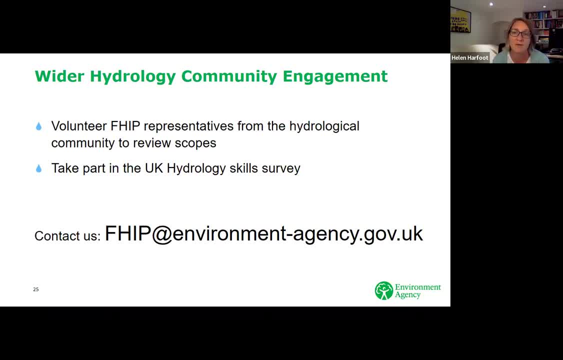 think it's just the start of the discussion on uncertainty, and there are projects that follow on from that which may result in in updates to the guidelines and the modeling standards. great thanks, helen. um any any more questions from anybody, you can add them in the chat or feel free to raise your hand and we can come. come to you. 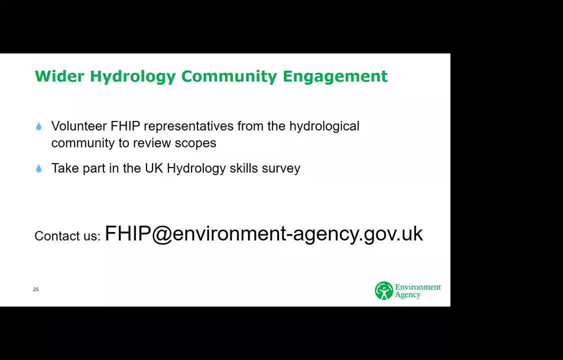 we had um a question earlier about um whether the powerpoint would be available, and just to note that the recording will be put on the um bhs youtube channel. but, um, i guess the team could consider whether they could share the slides on the on the bhs webpage which is will be coming. 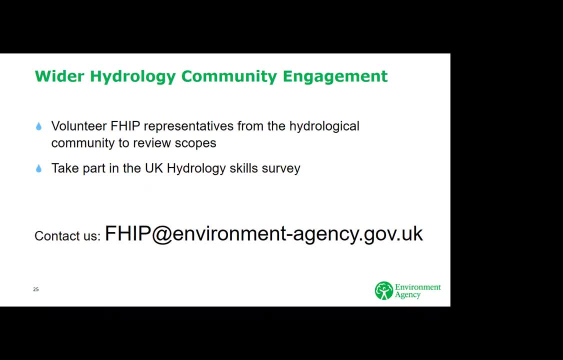 soon. so when that, when that web page there is there, we will um advertise that through the vhs website and we will be able to share the slides on the on the vhs website as well. so be sure to share the slides on the vhs website and we will be able to share the slides on the. 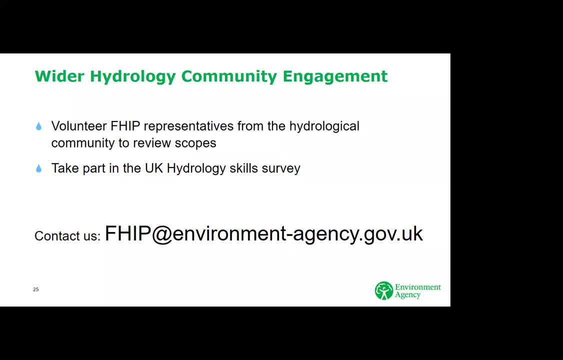 vhs website and we will be able to share the slides on the vhs website and we will be able to share them in the mail base and online as well. so just watch out for those those things when they're published. i have another question here, that from steve cole: will some or all of the fhip projects? 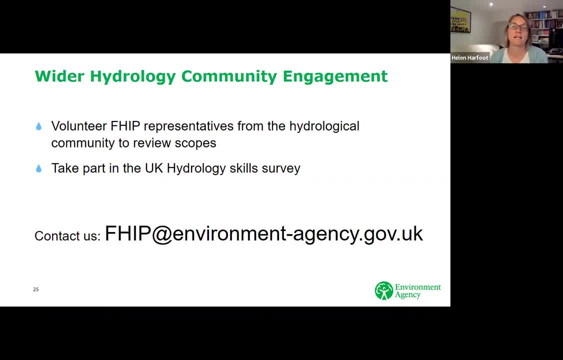 be open to the whole community to apply for or just advertise, through existing frameworks, future projects, and so I- yeah, I don't know, I can't answer that, but I think we would like to perhaps offer consultants or researchers outside of the normal frameworks, but no, we haven't made any decisions. sorry, I can't answer that one more clearly. 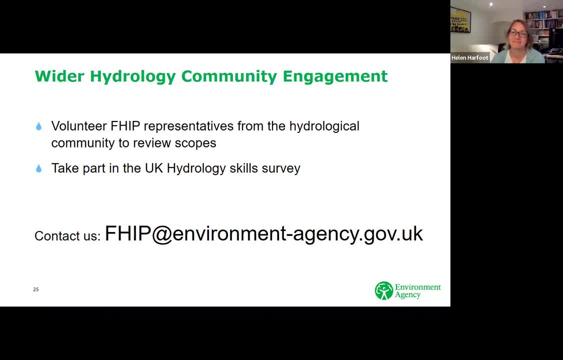 thanks for that, Helen. any other questions? so in in the chat. so in in the chat. Crystal has just commented, I guess, in response to that, that we'll have to strike a balance on that one and procurement and resources are in limited supply. so something to note. I'm thinking about the forthcoming, any forthcoming projects. 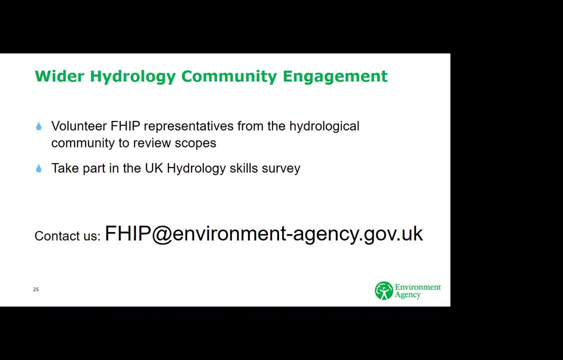 Nick, thank you. a question here for Helen. new catchment-based methods were mentioned. can you describe what this means by giving out proposals from S Council? is it bringing new methods out that are still in force? I think this is just really about bringing perhaps methods that are already in wider use, but actually just bringing them into operation. we're not looking to actually create a new method here. 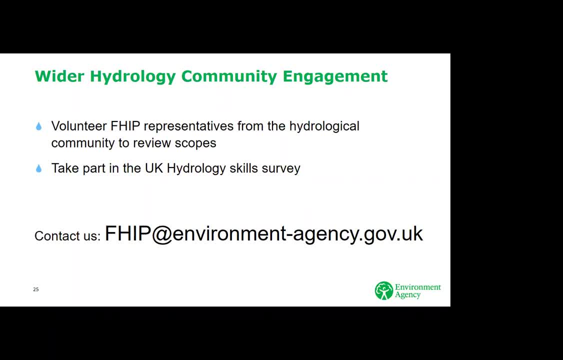 so this is just really trying to look at different ways of bringing different ways of flood estimation. So this is just really trying to look at different ways of bringing different ways of flood estimation. it meant more at a sort of catchment scale rather than individual site scale, or yes, yeah, yeah, that's. 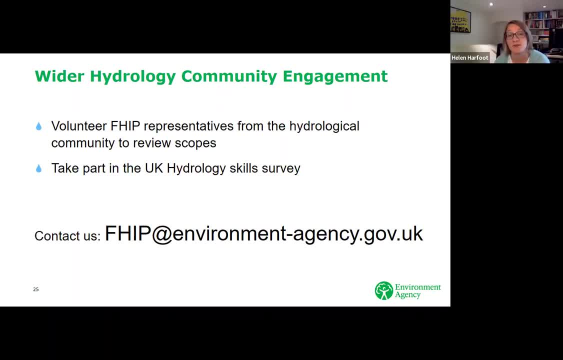 the intention, so um the vision of the 25-year roadmap is for kind of a more integrated catchment model. so we obviously don't have anything yet, so this is just really about looking how we can progress along that. that's that journey towards that long-term vision. okay, cool, thank you. 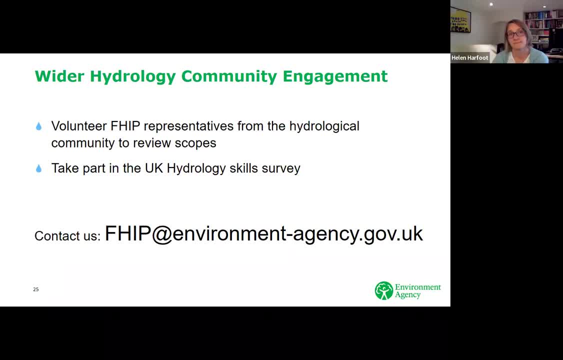 so it seems. it seems perhaps no more questions. um, i would just like to say thank you very much to um, hayley, helen and mark for giving today's um web bhs webinar.